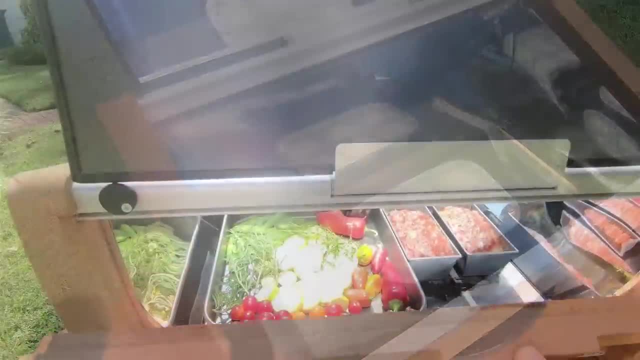 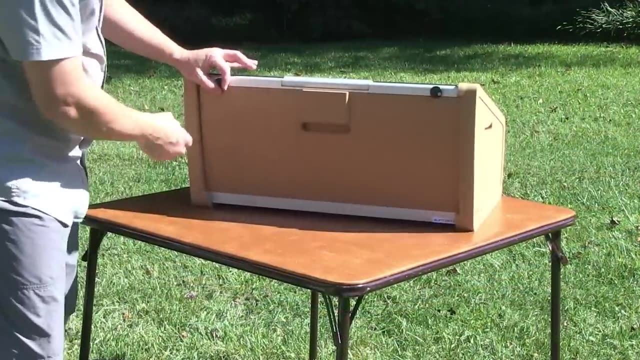 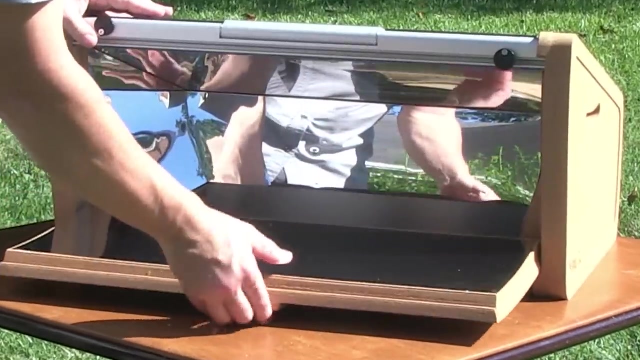 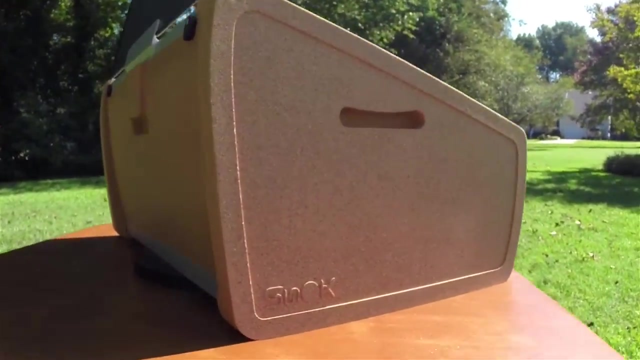 So it's been a little while since I've done a solar cooking video, but I wanted to put this one out there because I came across a solar oven that has really just blown me away. For the past couple of years I've actually been going over schematics and looking at drawings, at videos, on forum posts, Anywhere and everywhere I can find information on designing different types of solar cookers, especially the box type cookers. Not too long ago I was 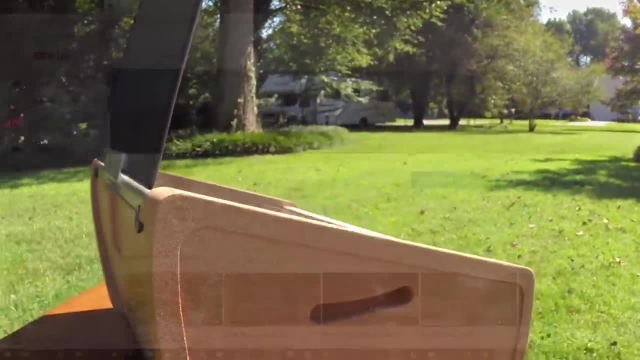 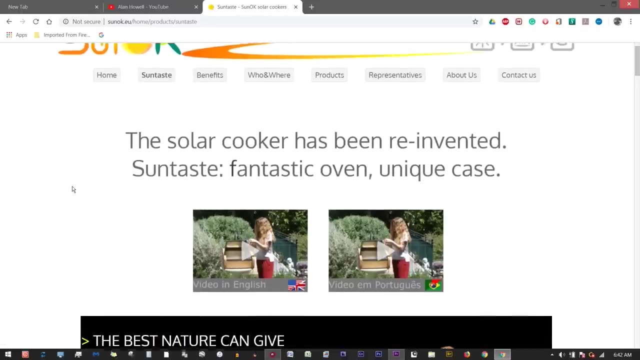 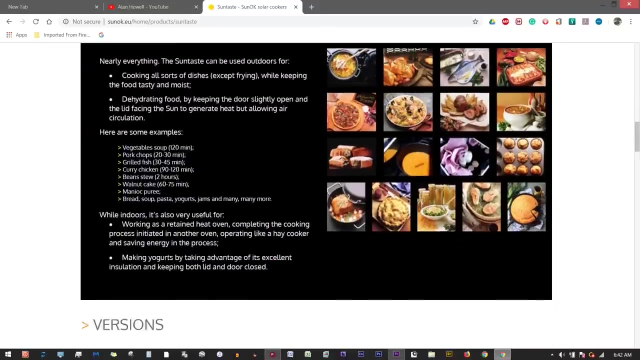 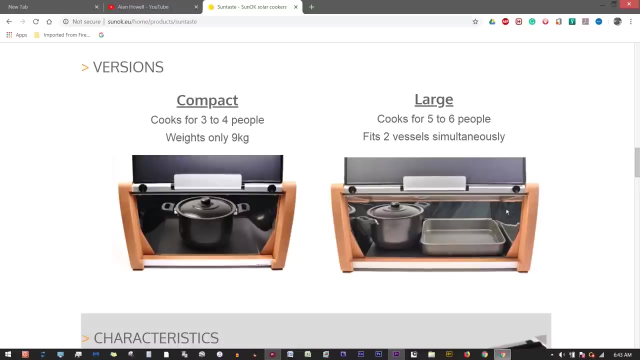 I stumbled upon the SunOK website. On their website, they have a solar cooker called the SunTaste and it comes in a couple of different sizes, But immediately when I saw this design, I knew that this was something I was going to have to investigate a little further, because the dimensions were very, very similar to what I was going to build on my own. However- and I have to give it to the engineers or the designers who made this- I 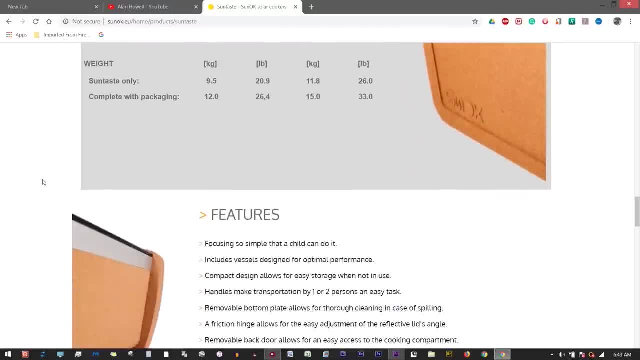 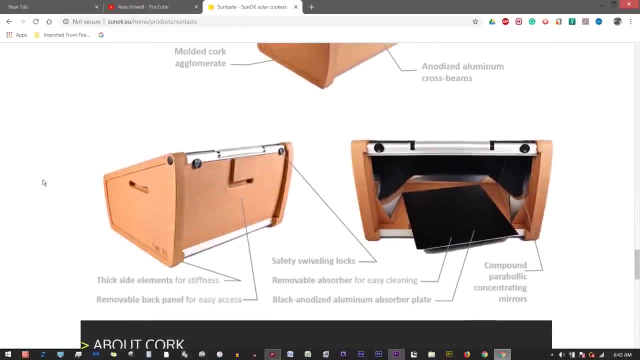 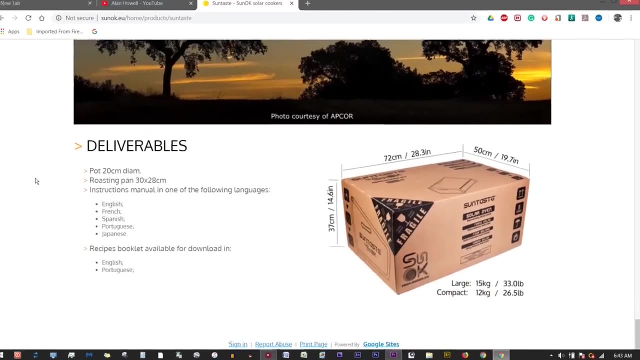 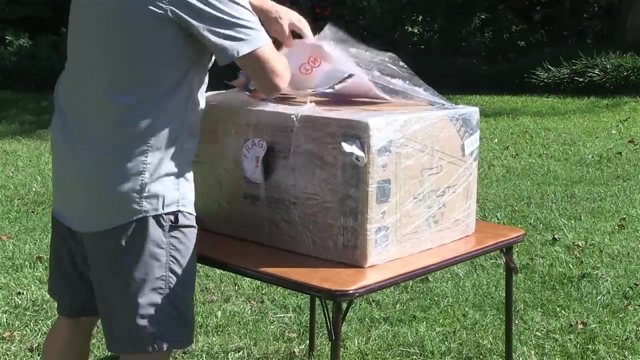 this SunTaste oven because they've taken it even a step farther than all the research that I had done by using cork as the main material that the oven is made out of It. just, it makes perfect sense to use cork because it is an extremely good insulator, It's fairly durable, It's not very permeable to liquids and things like that, And I did some research on this particular oven and I found out that they actually use 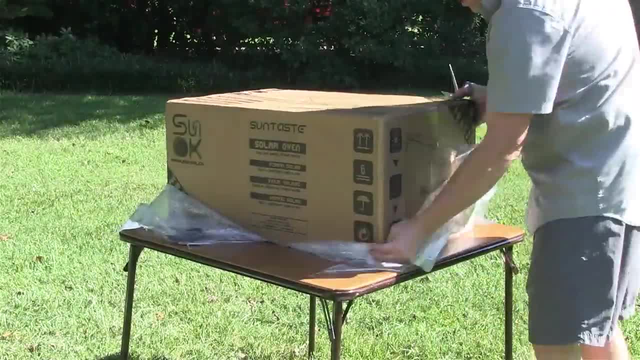 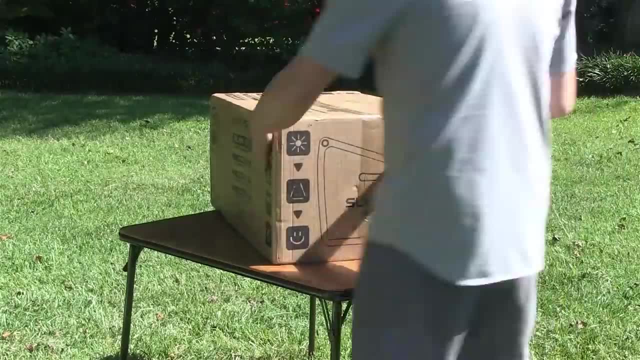 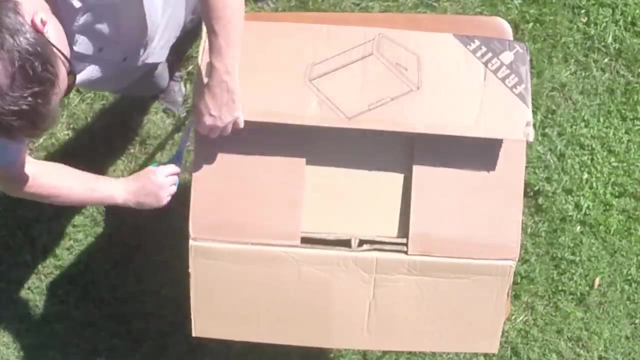 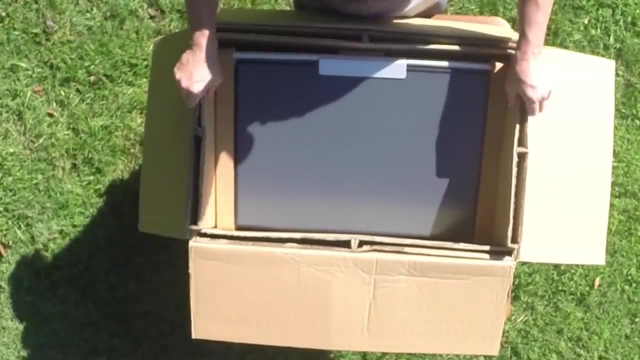 the actual raw cork material from the cork oak tree, which is basically just the bark of the cork oak tree. So what this means is that they're using cork that is a completely renewable resource. Whenever you take the the cork bark off of the cork oak tree, it does not hurt the tree. It continues to, you know, produce the cork bark. So this really just made a lot of sense, because one of the main problems that I was having with the 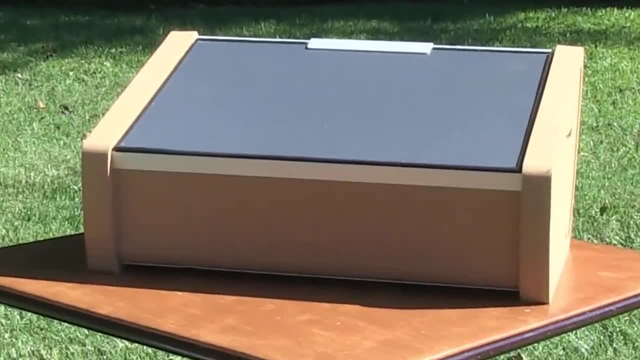 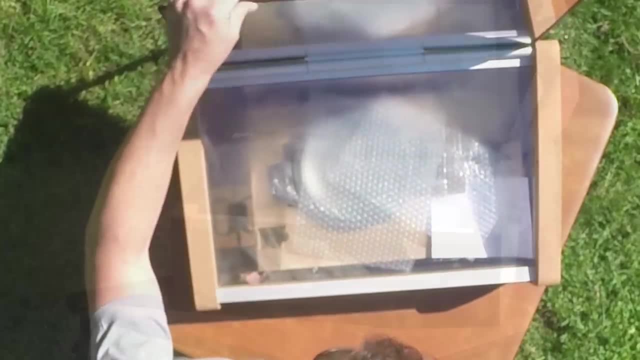 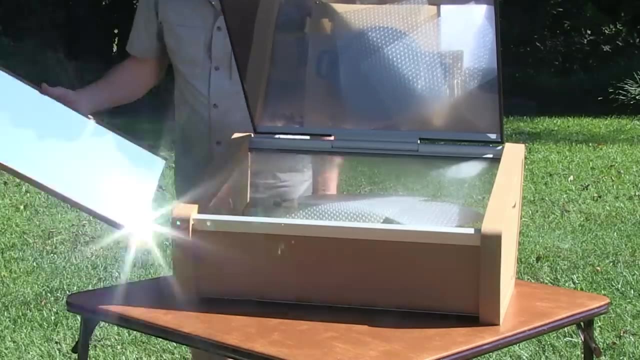 my designs is that they were pretty heavy. I think the lightest design that that I had come up with was probably around 50 to 55 pounds, and that's actually fairly light for a DIY type box solar cooker that you know, that is fully insulated, that utilizes actual glass. you know none of that. 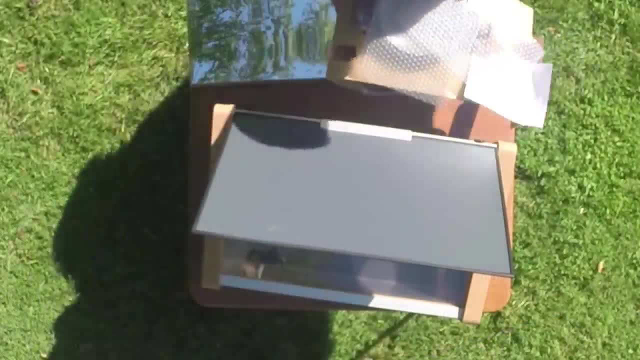 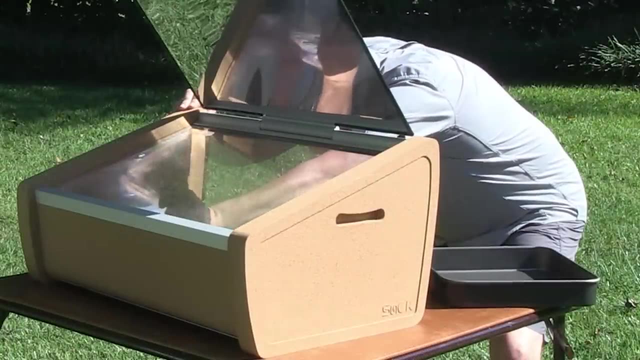 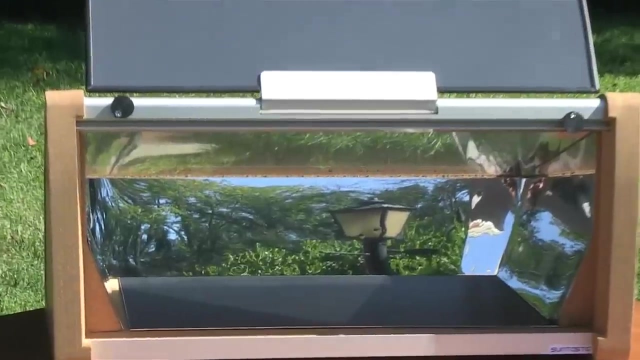 plexiglass stuff. So somehow they have been able to get this oven down to. it says on their, on their website, that it's 26 pounds. It honestly it doesn't even feel that heavy. I'm wondering if the 26 pounds is with the oven and the shipping box and materials and stuff like that as well. 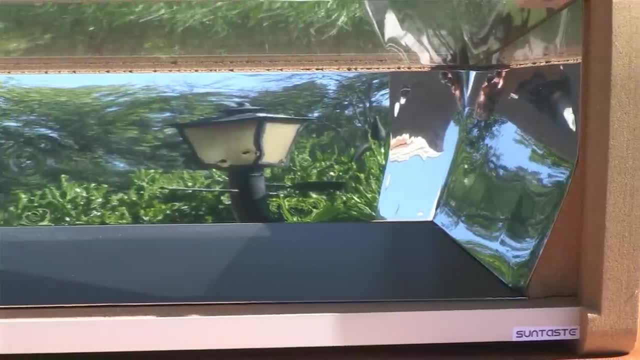 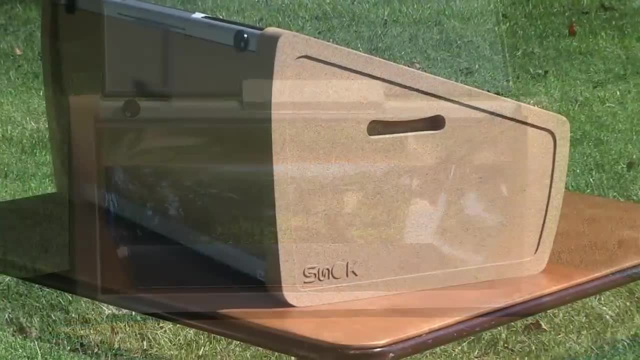 with all the things that it comes with, because it feels more about, like you know, 18 pounds to me, which is a really good weight because it's light enough to still travel, It's easy to carry in and out of the house, It's still got enough weight to where it's not going to. 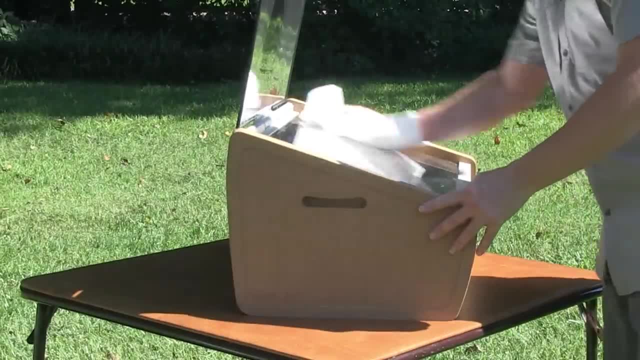 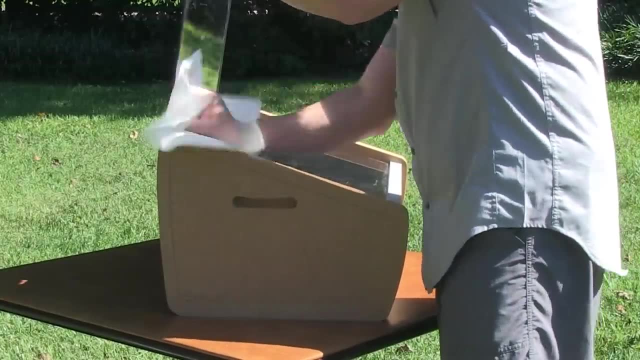 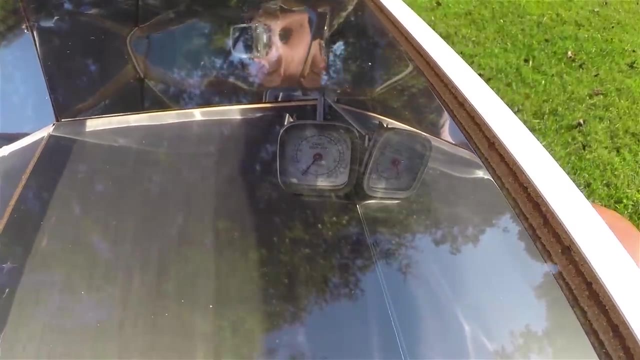 fly off the table outside in a good strong breeze. So, as you can see in this, in this unboxing, it does come fully assembled. The only thing that I had to do was just basically peel off the plastic protective covering over the reflective surfaces and I just kind of gave it a quick wipe down. 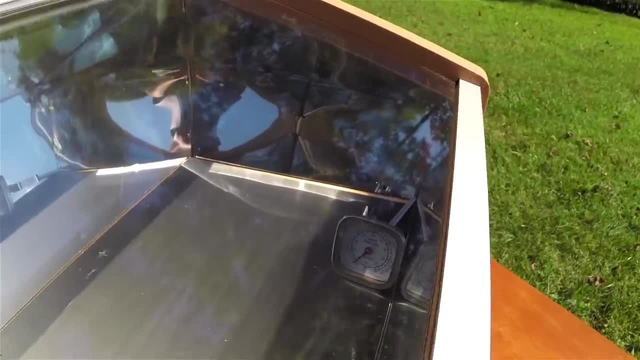 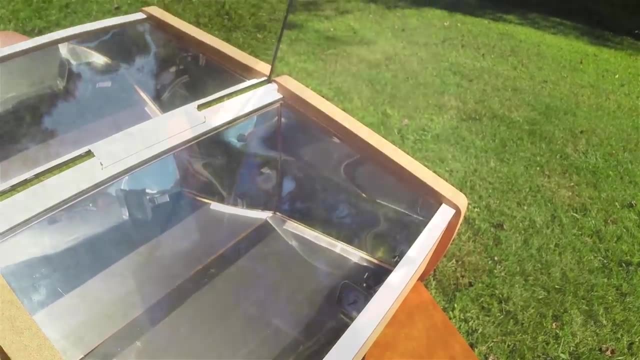 Just, you know, brushed out any, any dust and any of the fingerprints and stuff on the glass and reflective surfaces just to make sure you're getting the most efficient heat transfer. and I was up and running, I was up and running, and I was up and running, and I was up and running, and 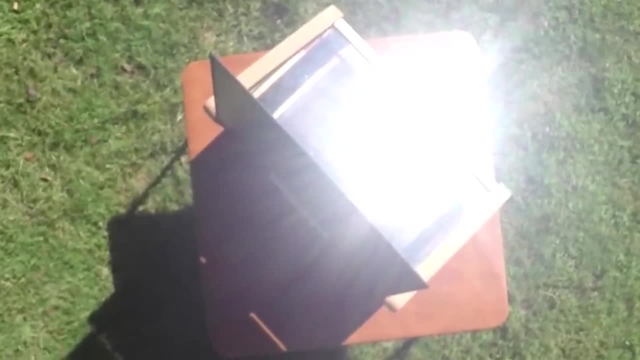 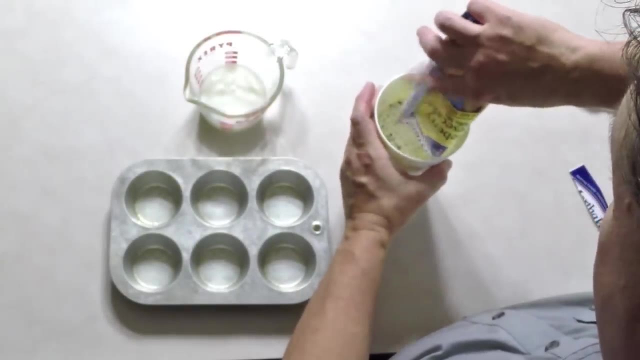 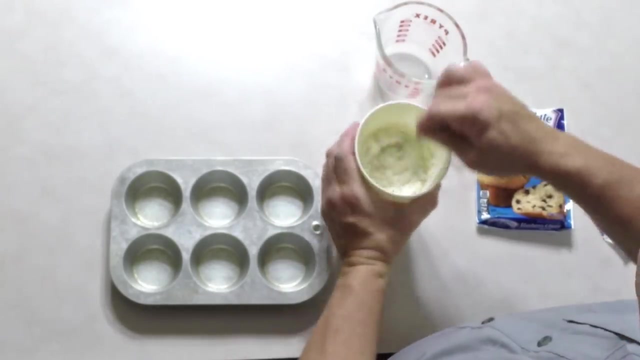 running in like 15 minutes. I mean, I was just blown away at how fast that. you know you can be cooking with this thing. Normally when I do solar cooking it takes me about, you know, a half a day to kind of prepare. I'll decide on what recipe that I'm going to do, The first thing that I usually go. 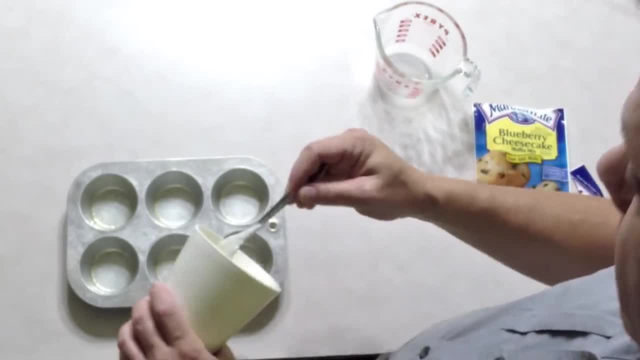 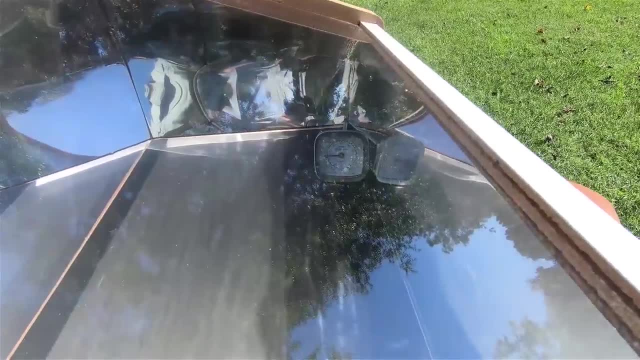 So, anyway, I picked up the large version that they sell, which is said to basically cook enough food and have it cooked. I don't know if it's going to be good or not. I don't know, I don't know, I don't. 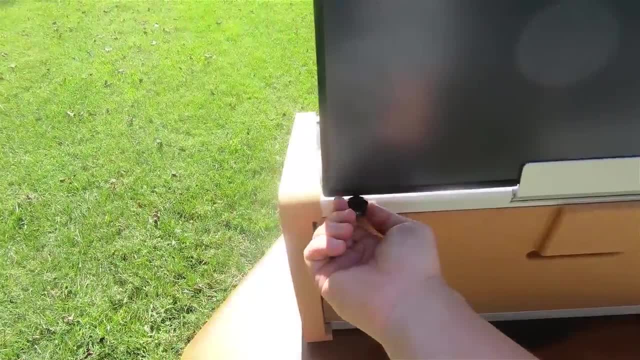 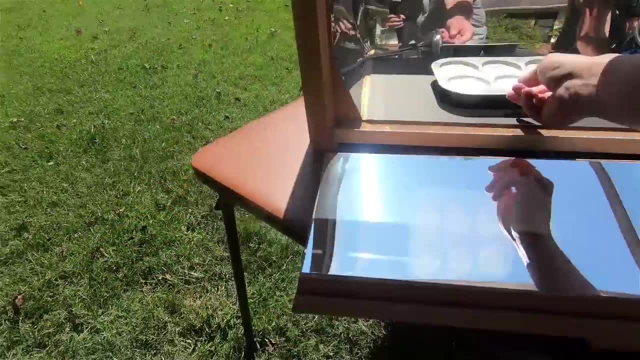 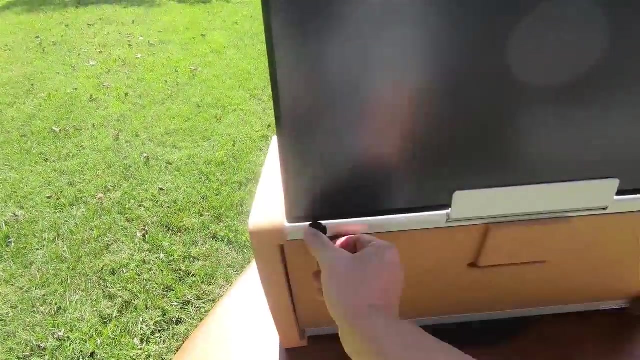 in one setting to feed five or six people. The amount of food that you can prepare in this is is really, really amazing. To be perfectly honest, I really don't like unboxing videos, but I did want to do this, just simply to show you. you know what, what comes with the, the oven, and that it is. 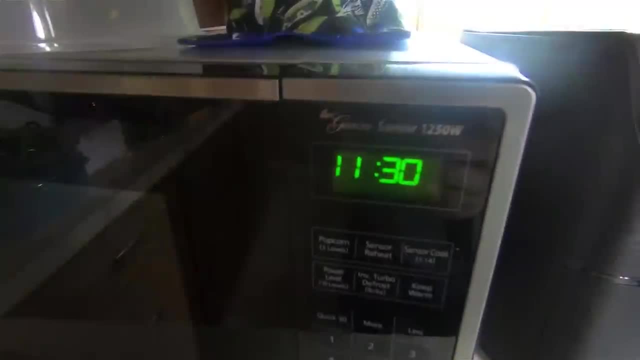 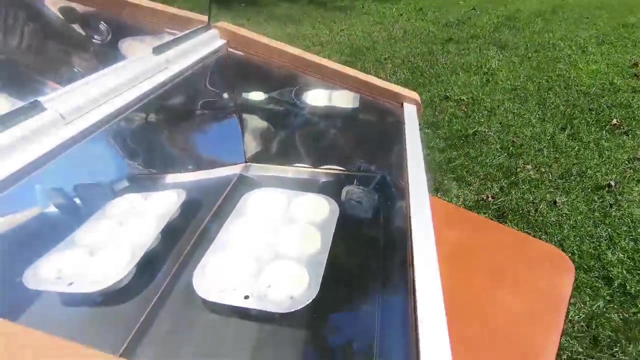 actually delivered completely assembled. That was the the first surprise that I got when I received this, because I fully expected to have to, you know, at least put some money into it. But when I got to the restaurant it was really amazing. I mean, I was like what is this I'm going to do? And I was like 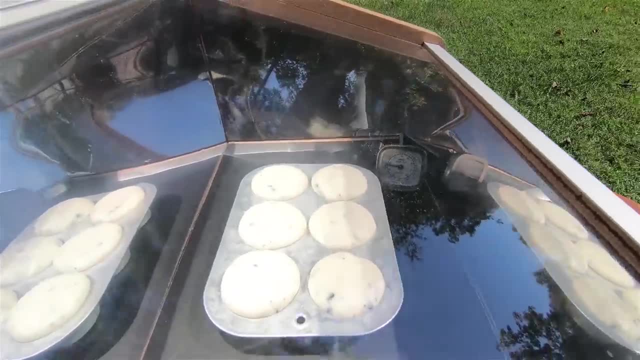 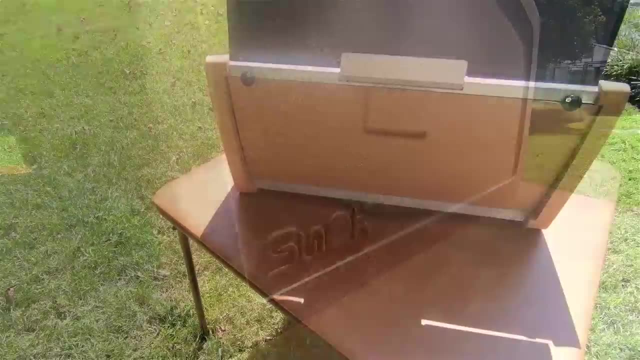 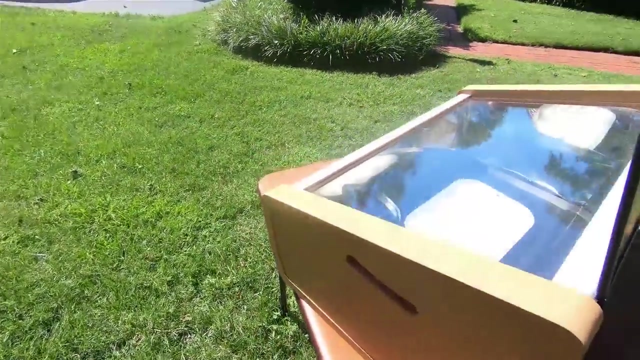 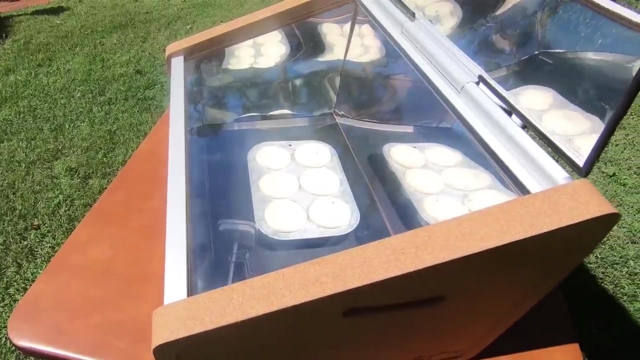 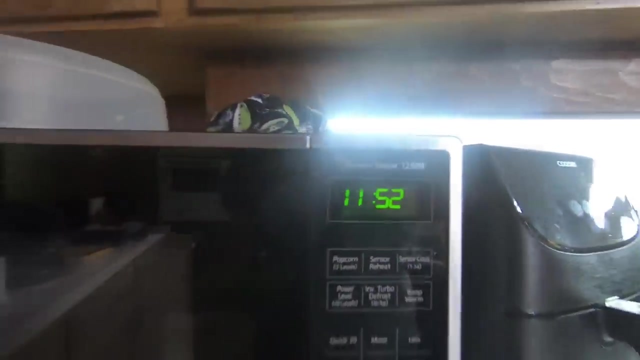 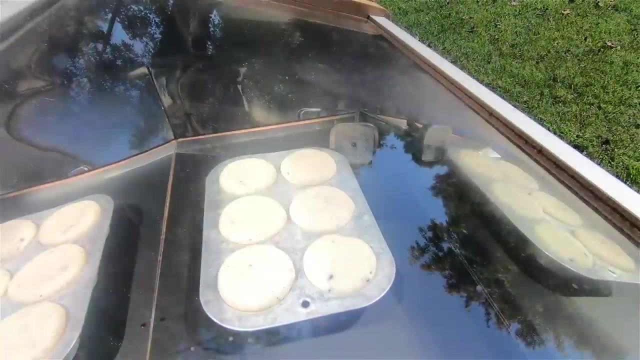 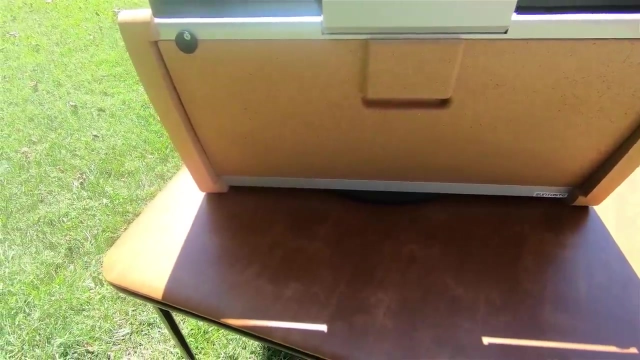 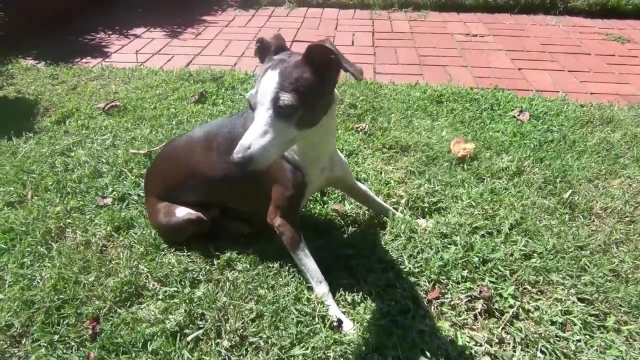 parts together. you know, maybe lay the glass in, even, you know, just the absorber plate in the oven, whatever it might be. but this thing came completely assembled. not only that, it actually comes with a really nice roasting pan, and flavors just seem to blend really well. it seems to benefit from the, from the 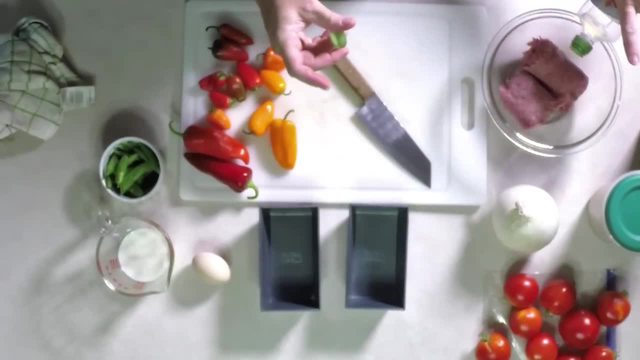 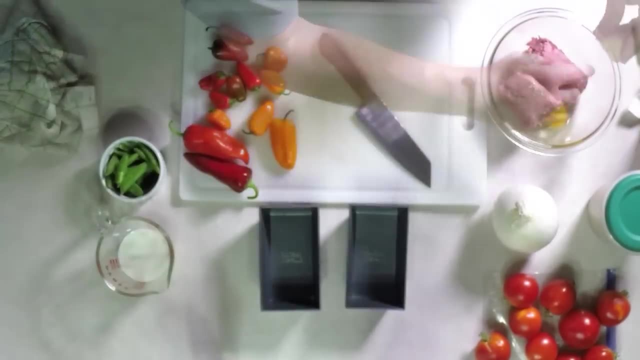 longer cooking times. so here I'm going to show you how I put together my meatloaf for solar cooking. just a pound of hamburger coat, that with a little bit of light olive oil, and then I crack either one or two eggs on top of that. add a few bread crumbs to it. 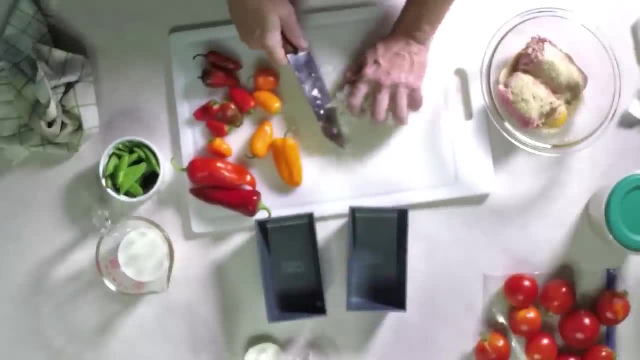 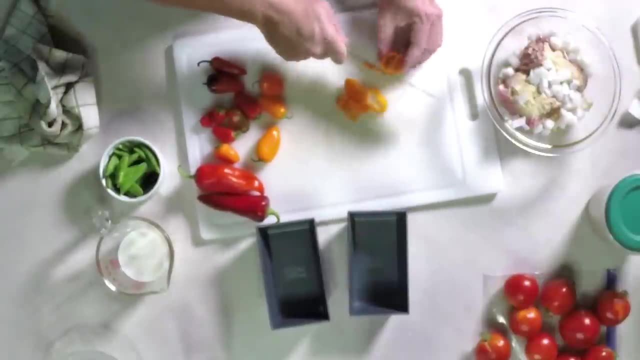 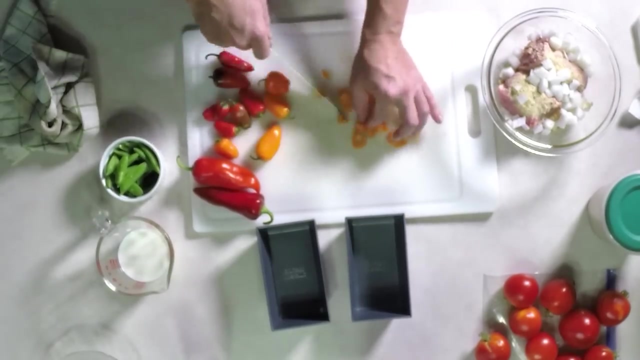 those are like the seasoned bread crumbs, a little bit of onion. and then in my garden I raise sweet peppers and hot pepper, so I add some of my favorite sweet peppers. this pepper is called a yummy orange sweet pepper. these are really really superb, highly recommended. and then I add some red. 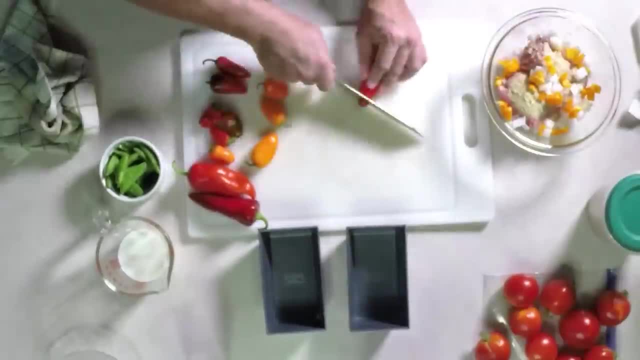 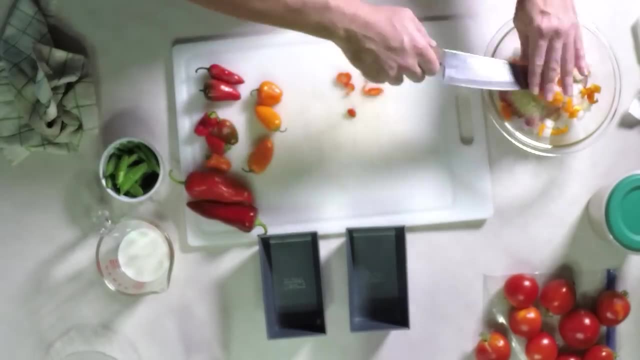 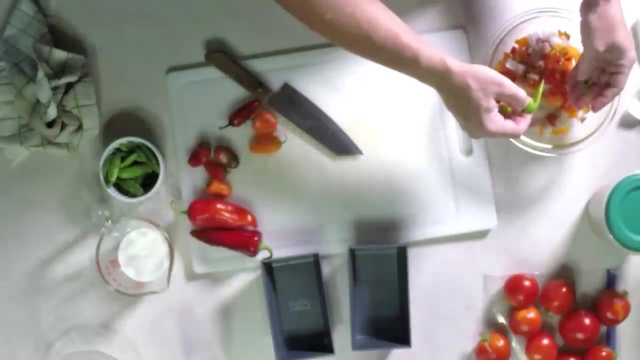 what's called lunchbox peppers, which is also a sweet, a sweet pepper. the peppers really add a nice flavor to it. and then I get fresh sugar snap peas and I take the peas out of the pods and I put the peas into the bowl. makes a huge difference over just using like canned peas. 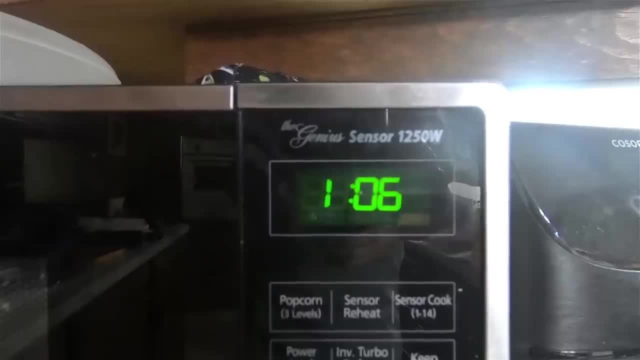 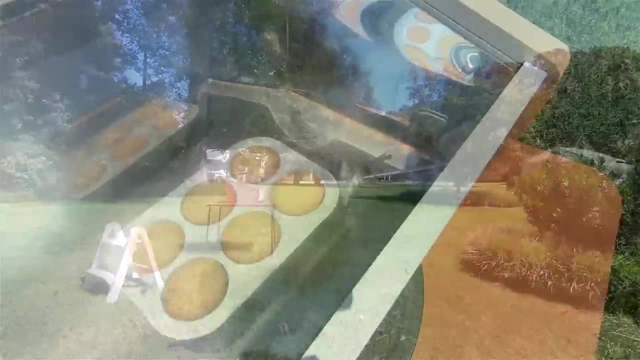 inside your abrirts meatloaf and cook it in the brain for another 12 instant or 20 minutes, right before I put one into the frying pan. so you also have to set the heat on high every now and then. I would check on the, the muffins and 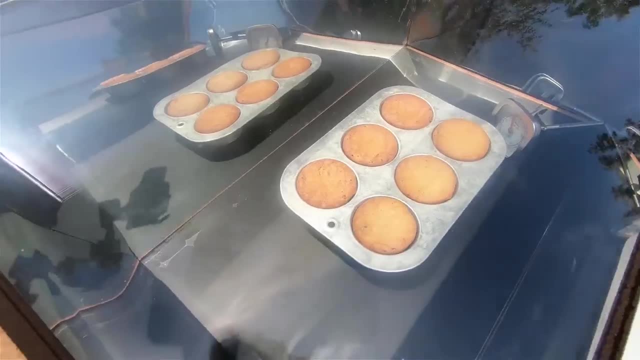 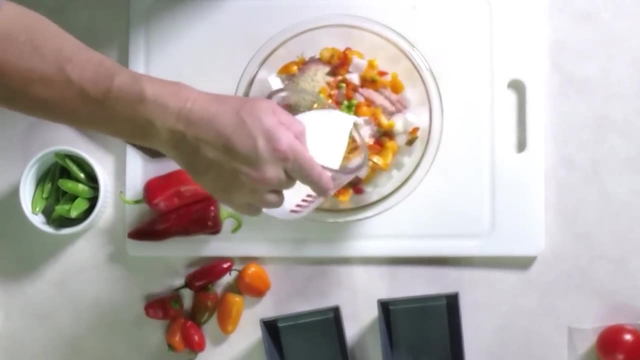 this was probably the point I should have. should have taken the muffins out. they were already done and I thought: well, I'll just leave them in just a little bit longer, you know, while I'm finishing up the meatloaf. that was my mistake, I should have went ahead and taken him out, but anyway, so I had a. 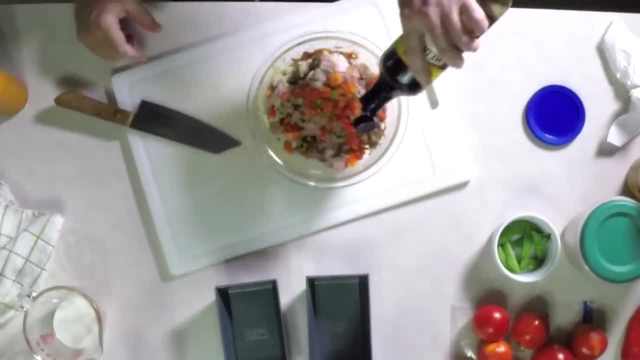 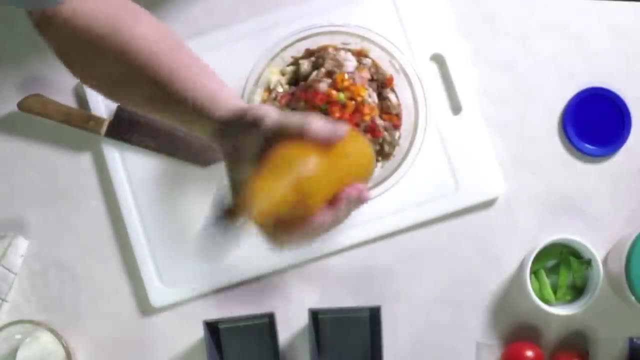 little bit of milk to the mixture and I fold that in just kind of a few more bread crumbs there and that was pretty good, and then a little bit of Worcestershire sauce And then I add: this is my own making, this is a Caribbean-style mango scotch bonnet hot sauce. 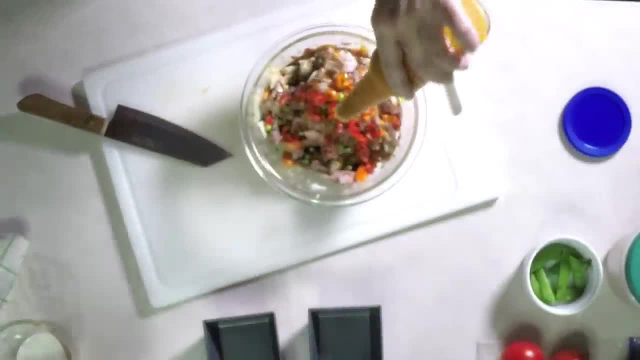 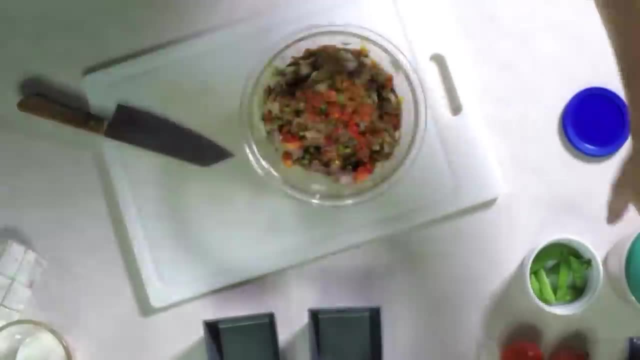 which is just phenomenal. It's got a little bit of sweetness and quite a bit of heat, A little bit of brown sugar, maybe just like a tablespoon or so of brown sugar, And what this does is it helps blend with the sauce that I put on top of the meatloaf. 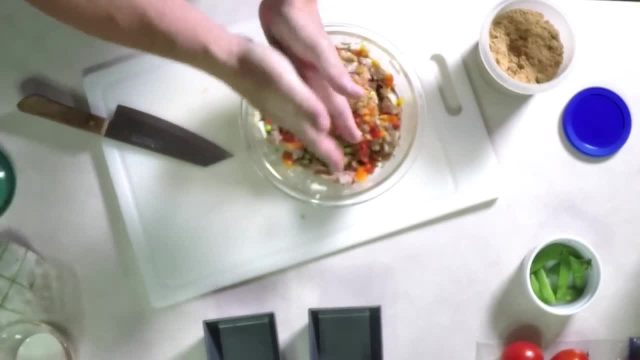 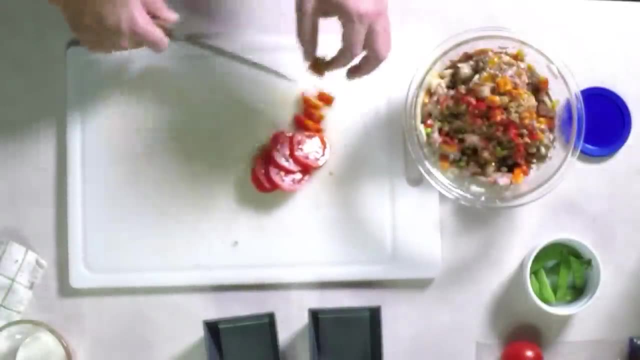 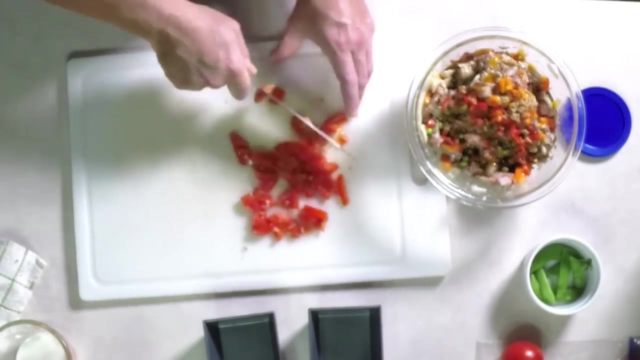 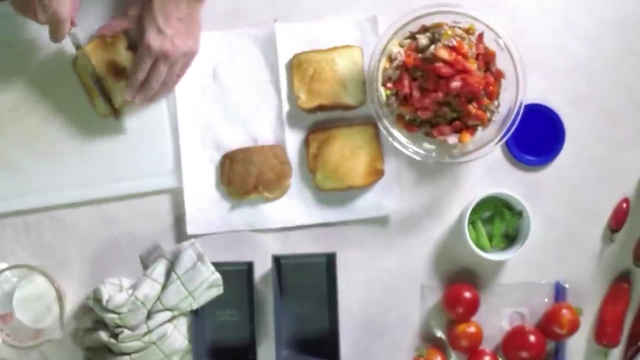 I'll dice up a few small tomatoes and add that to the bowl, And then I'll make some toast and I'll dice up the toast and add that in. Add that as like an extra breadcrumb or something like that, And then I'll add the rest of the sauce. 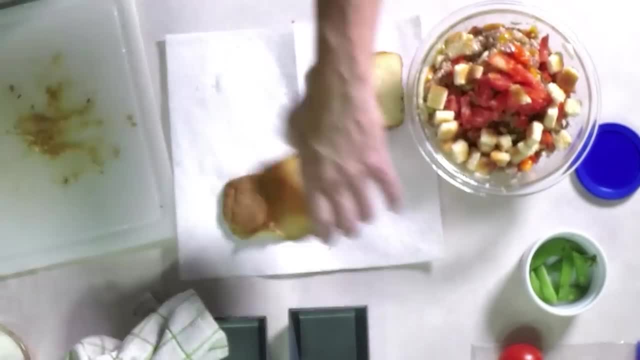 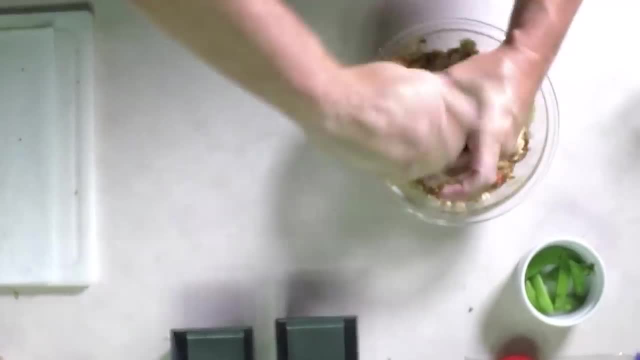 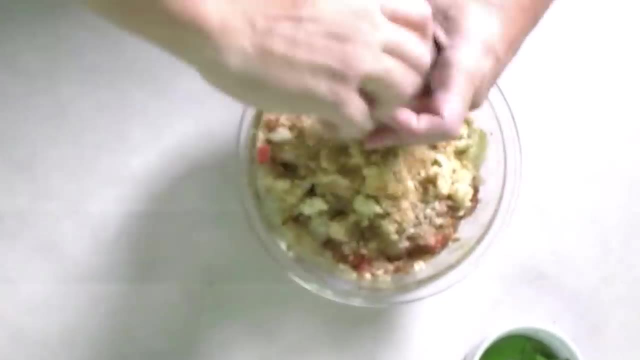 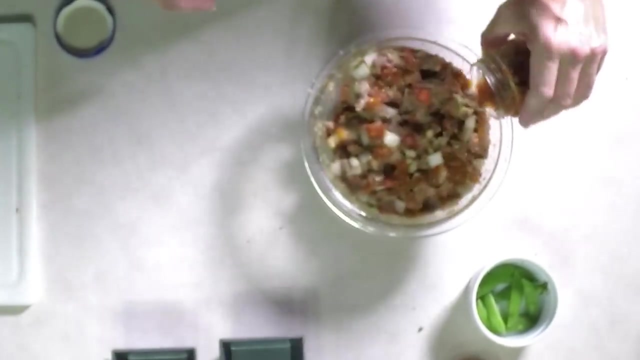 It's more of a texture thing, And then I'll add a little bit of salt and pepper, And then I'll add a little bit of salt and pepper, I'll fold everything in- Try not to overmix everything- And then I've got a little homemade salsa. 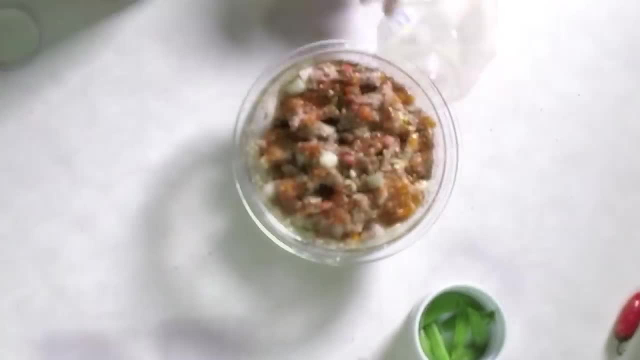 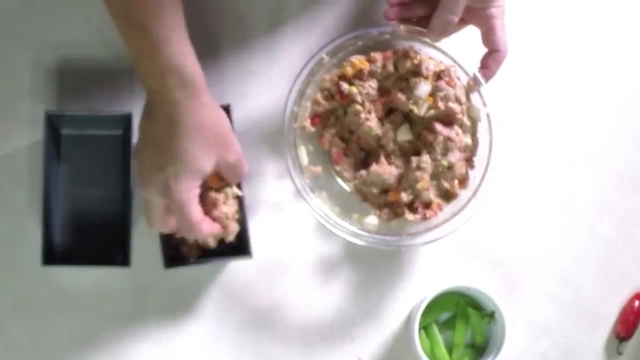 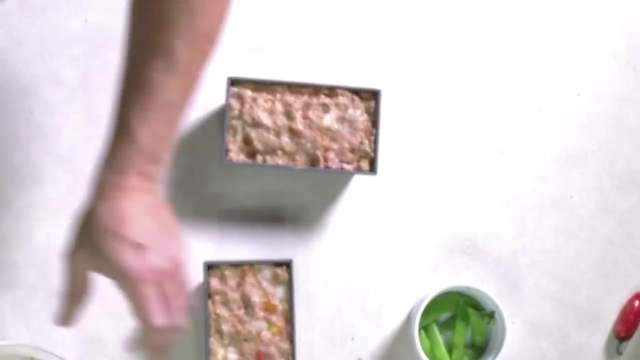 that I mix in there as well. That's obvious, because when it's justagenese, that's, you know, obviously optional, that the hot sauce and salsa is obviously optional. so I'll load this mixture into these, these small little loaf pans, and that seems to be the the perfect size for making like a meatloaf. that would. 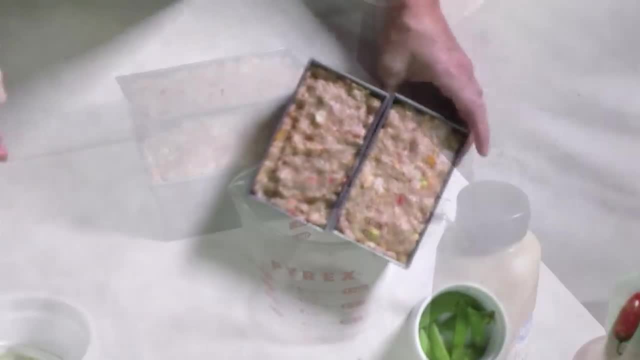 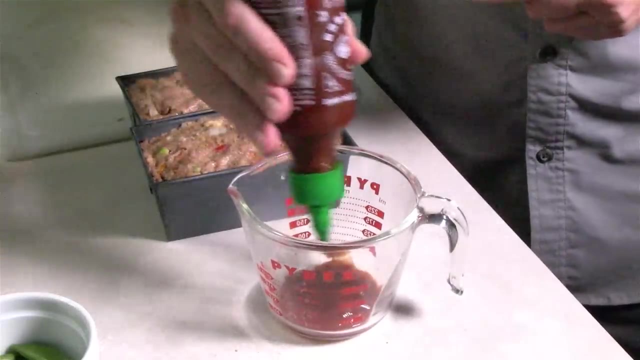 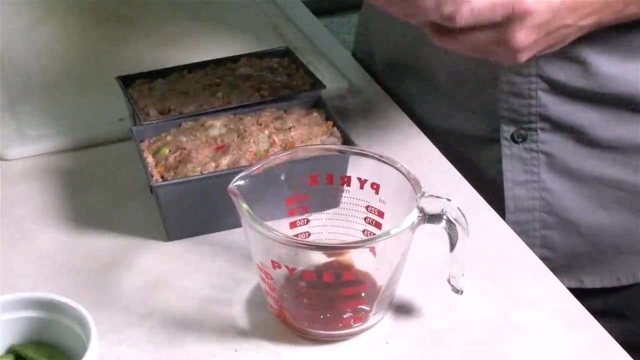 would feed about two people. so for the sauce on top I add a little bit of ketchup, some sriracha, and then I'll add some, some honey, Dijon mustard and blend that as well. sometimes I'll add in a little bit of brown sugar to this. this. 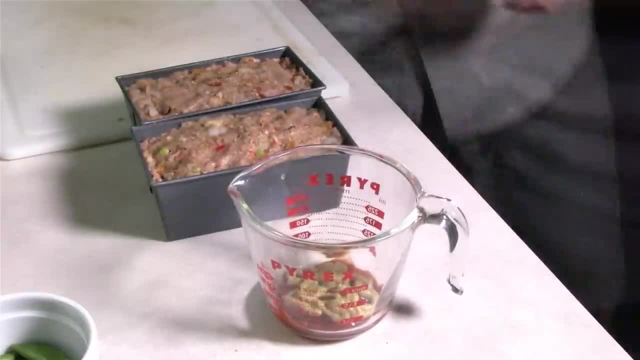 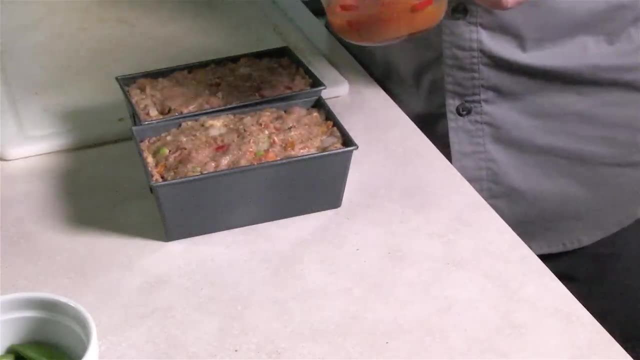 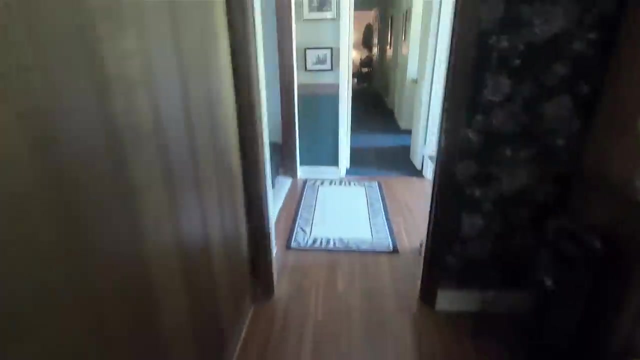 part as well. it helps the caramelization and the glazing process. I'll put the meatloaf in the solar oven, let it cook and let it brown, and I like to let it brown before I add the sauce on top. you can add more sauce if you want, but I like to let it brown before I add the sauce on top. 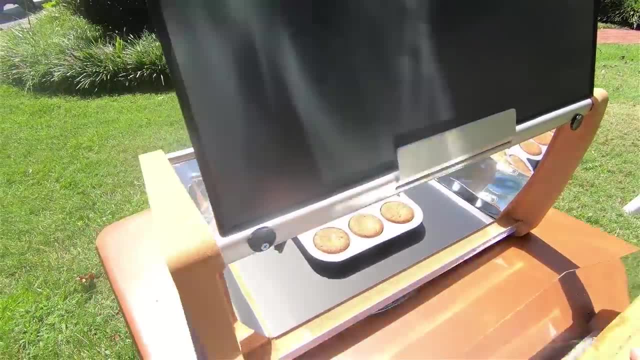 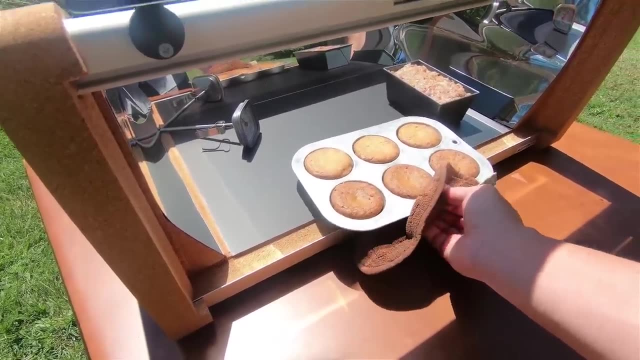 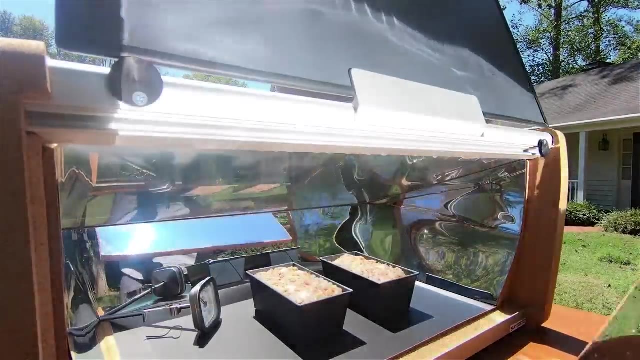 so here I'm taking out the muffins and, yeah, I got him a little bit overdone, so I put in the meatloaf and I actually had a thermometer inside. the temperatures didn't seem to be right and I noticed I moved the thermometer a couple of times and it changed the temperature drastically. so I think what? 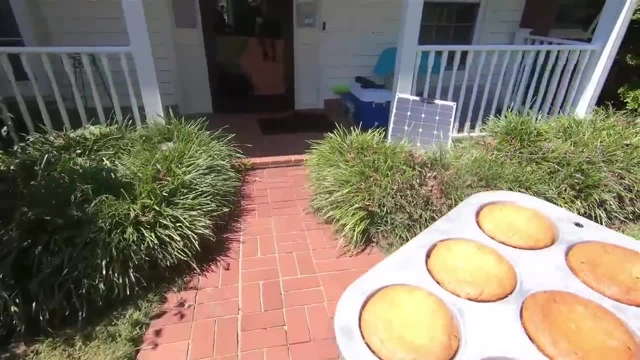 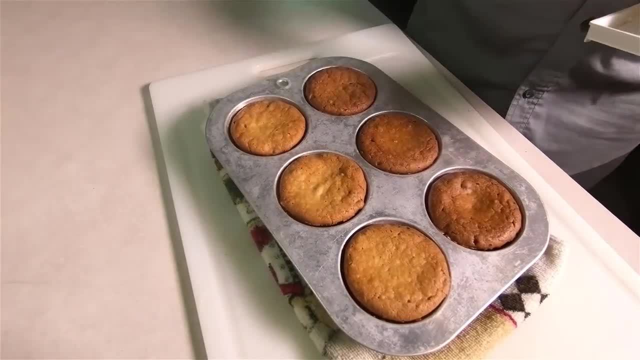 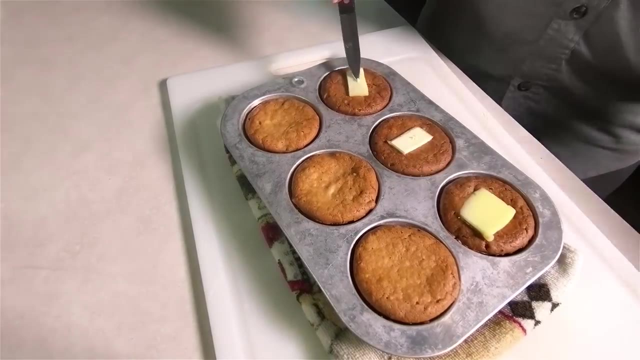 was happening is I was getting some Sun reflection spots onto the thermometer sensor itself and it was making the readings go go way up. it's my estimation that this particular day, I was getting anywhere between like 225 to maybe 235 degrees, which is actually the range that I look for to cook most of my 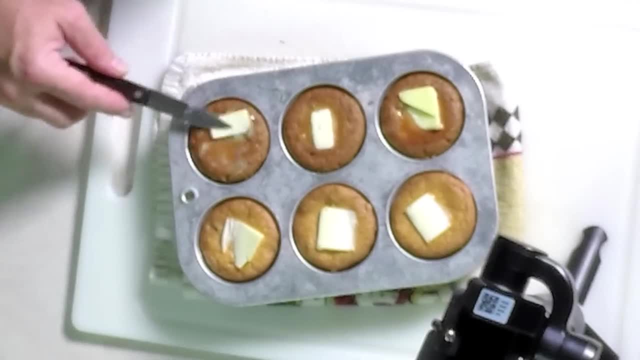 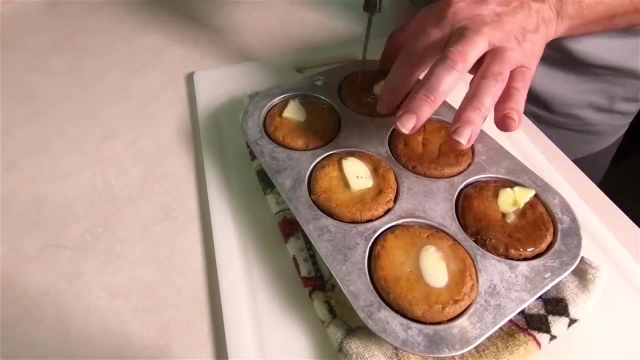 foods. now, if it's like a stew or something that I really want to do like a slow cooker process, you know, just barely over 200, I think, is really optimal. that way you can let it cook for four or five, maybe six hours and it really benefits that. the taste benefits from that slow cooking, slow cooking. 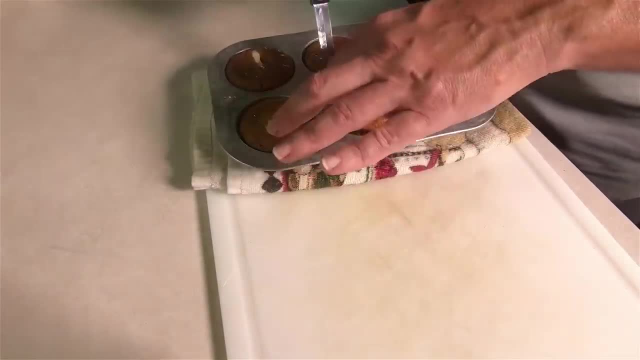 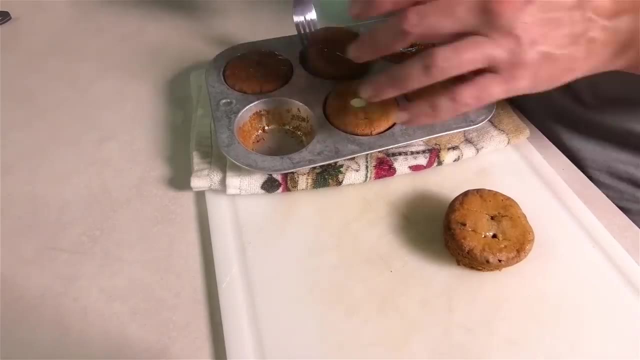 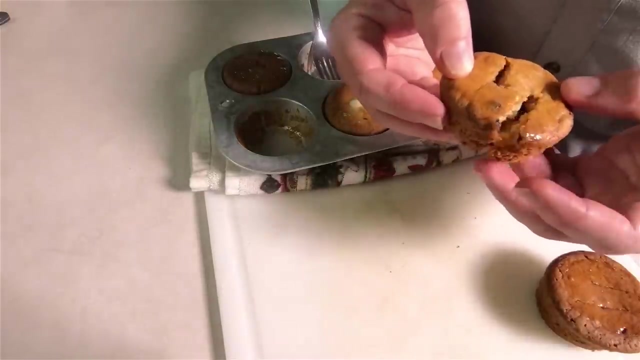 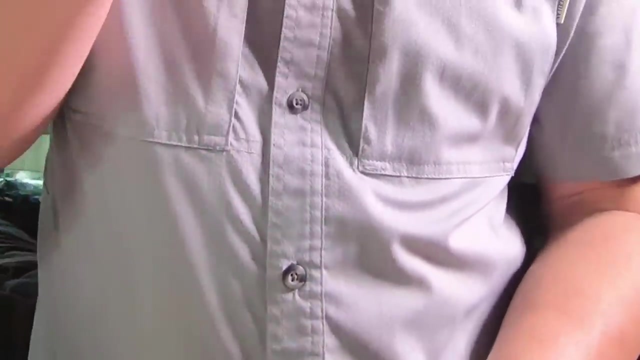 process. but these, these muffins, even though I browned them just a little bit too much, they were still really really good, especially when you you melt that butter into it, like that. I really really like it like that. you, you, you, you, you is that it never really like burns it. you can kind of overcook it, but it won't. 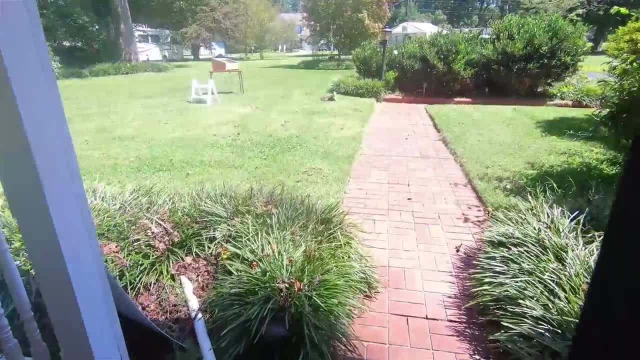 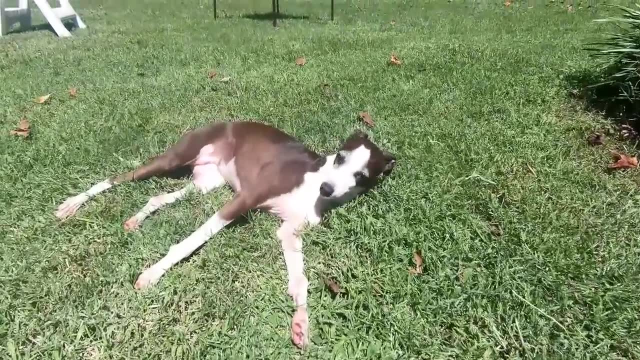 ever burn it so you don't. you don't lose the food. this is my dog, Thea. she, she's always around me whenever I'm cooking. she, she knows she's gonna get a little bite of something that that I'm cooking, so she's ever-present. so all I would 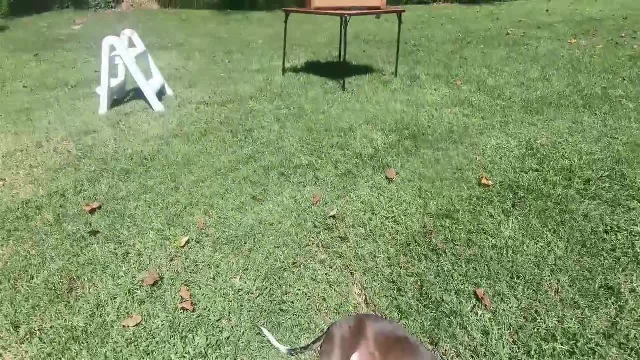 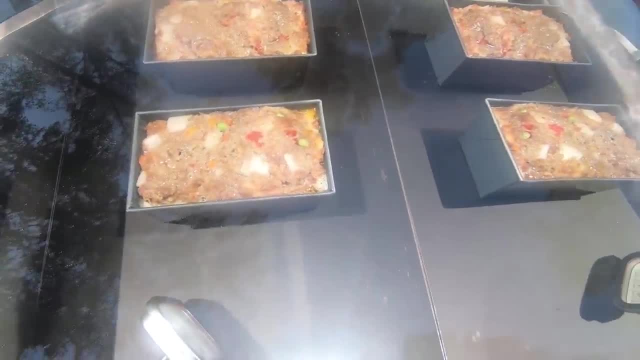 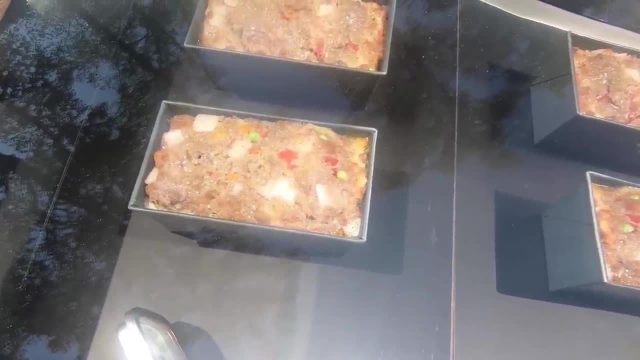 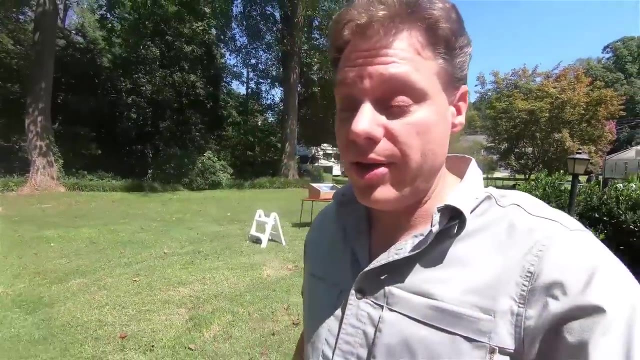 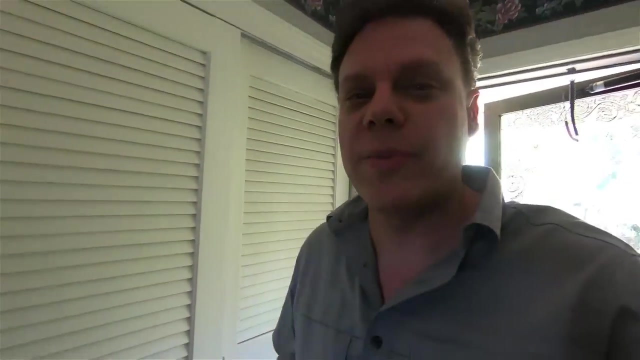 wanted to reduce the temperature a little bit. you know you just don't rotate it, and that way you can provide more of a slow cooking process that's not going to get too hot. it's gonna be good. I can already taste it. this is probably one of my one of my favorite meals. this is gonna be a real treat. 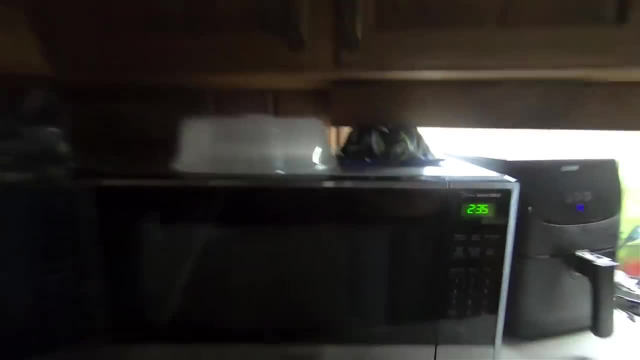 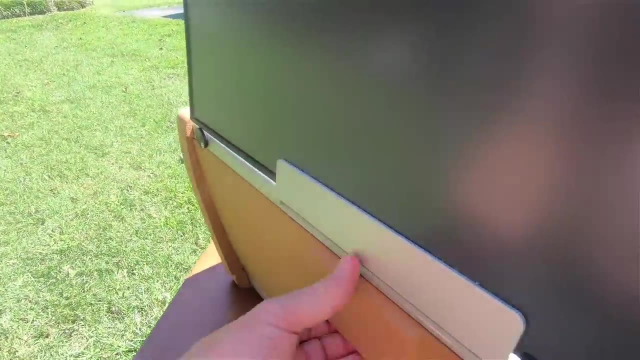 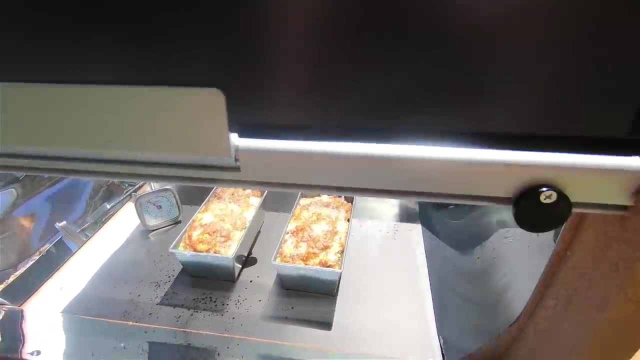 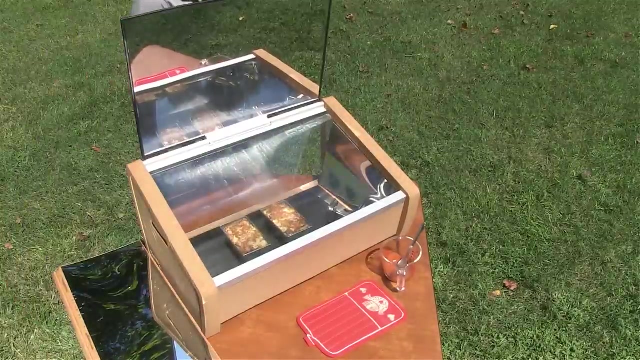 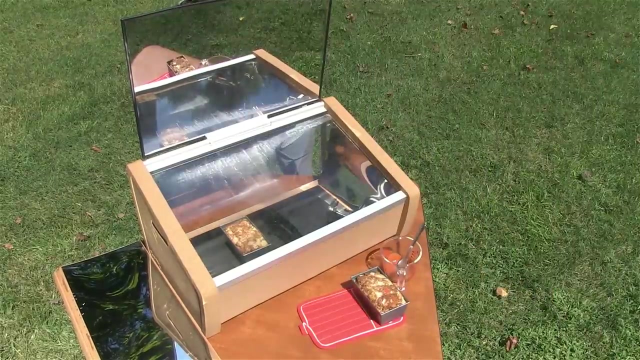 tonight you, you, you. so here I was checking on the the the browning process of the meatloaf and it it's just right. so I'm gonna take it out. and this is the part where I add the sauce to the top. if you add the sauce too early, it takes too much of the liquid. 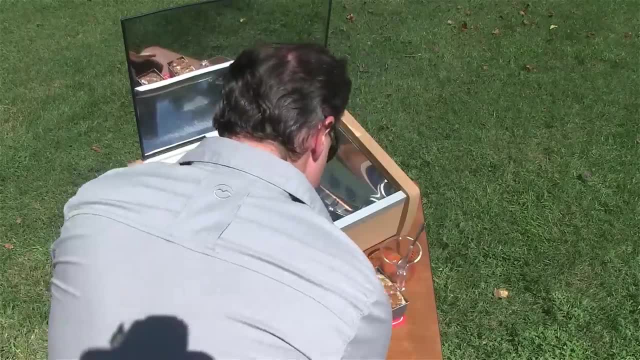 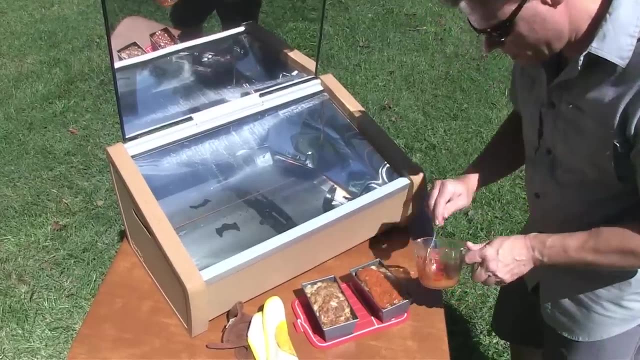 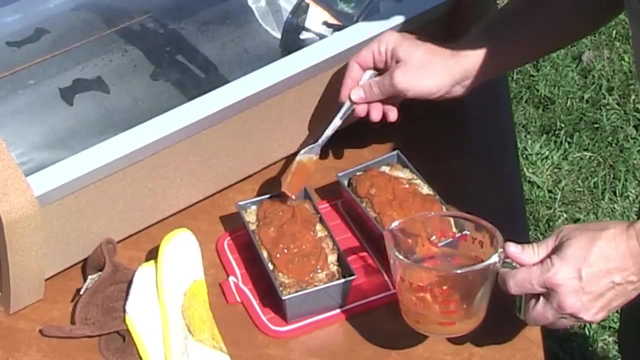 out of the sauce and it becomes, I don't know, almost like a like a rubbery feel on top, and then you don't want that. so you add your sauce, you know, laid into the cooking process, and this is just really a nice finishing touch to the home, to the meatloaf. it adds just a. 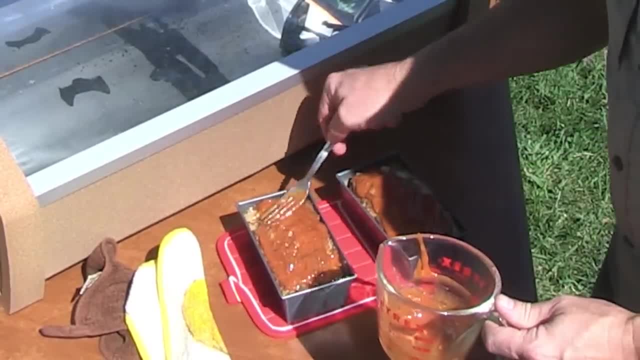 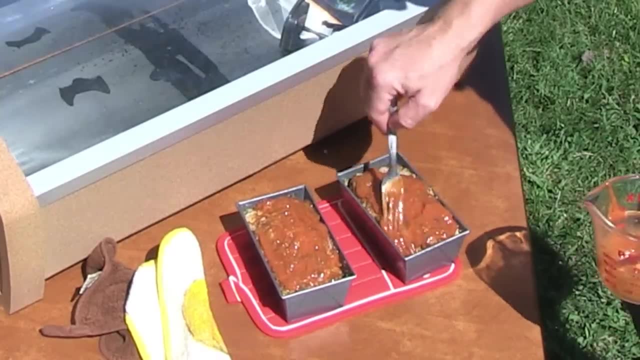 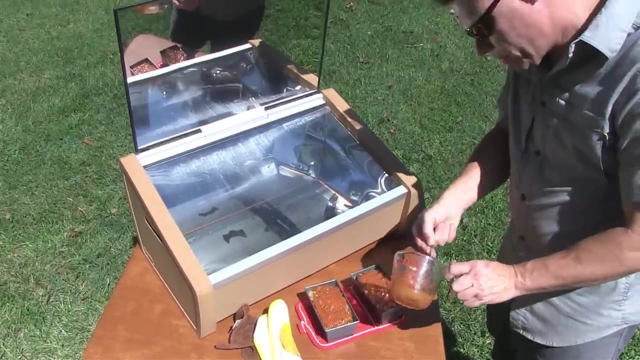 little bit of spiciness, you know, with the, the mustard, and that blends really, really well with the, the hot sauce that I add to it, and a little bit of the salsa inside you, you, you, now, of course, you don't, you know, you don't have to add, you know, hot peppers. 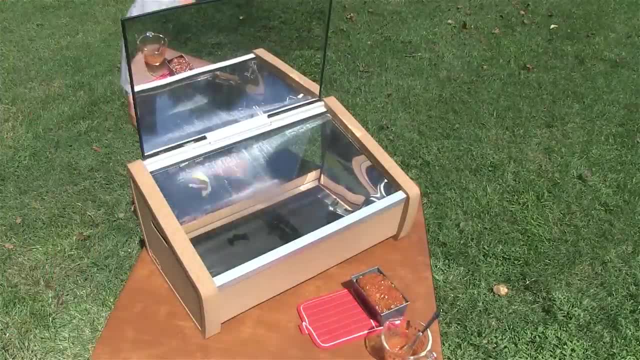 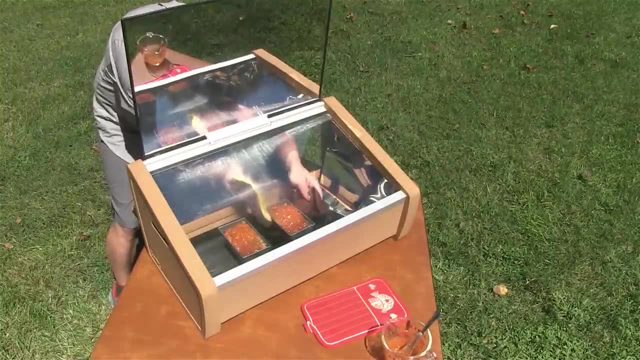 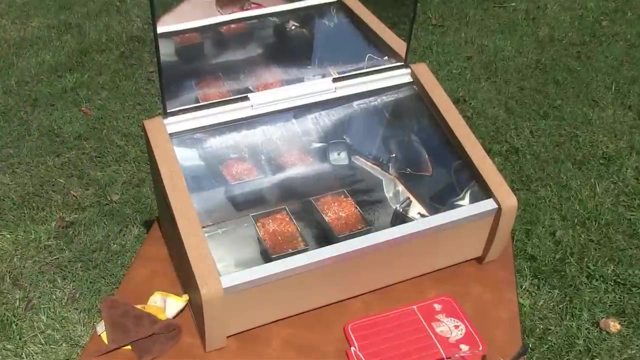 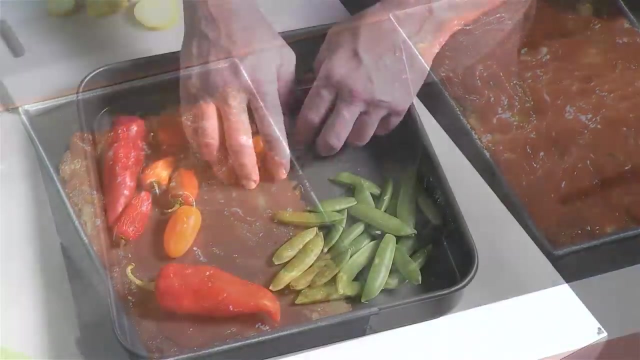 or, you know, hot sauce to the meatloaf. this is just my preference. I do highly recommend adding just a little bit of spice, though it really seems to make a meatloaf that that most people seem to enjoy. then I decided to go ahead and roast some vegetables as a side dish, and I 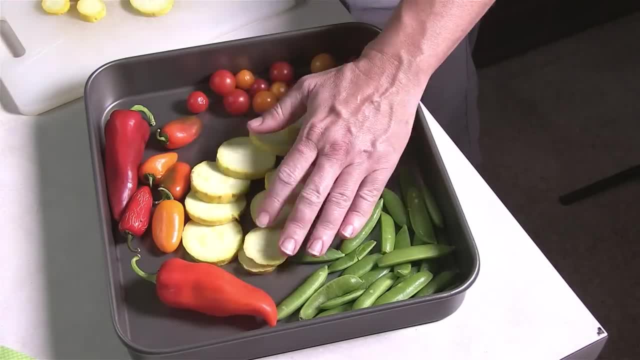 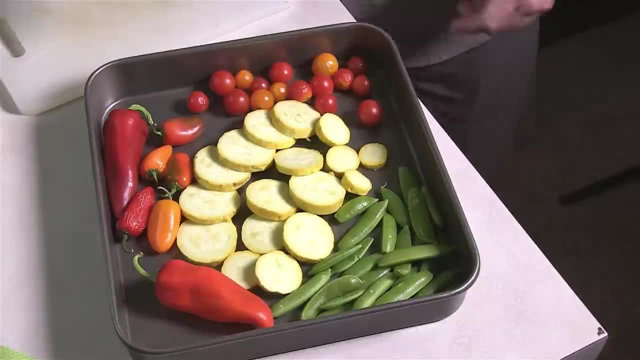 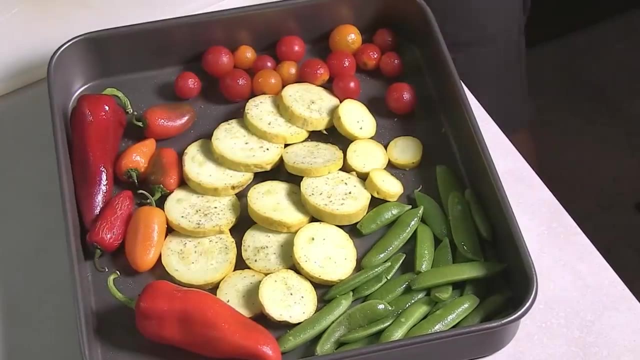 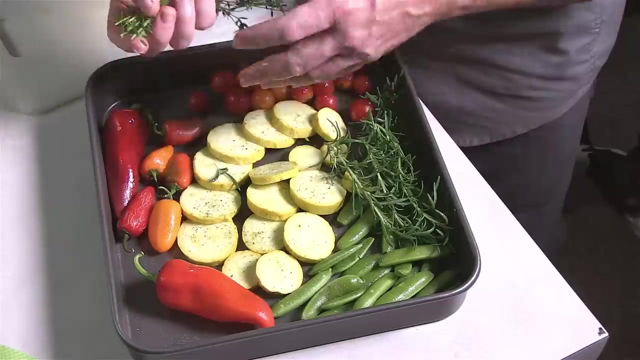 so I'll just put in some squash and some little cherry tomatoes- like three different types of cherry tomatoes, three different types of sweet peppers- think of chipotle pepper- and some sugar snap peas, and I also add in a couple of my favorite herb bundles I like sometimes. I'll dry out the herbs at the same time. 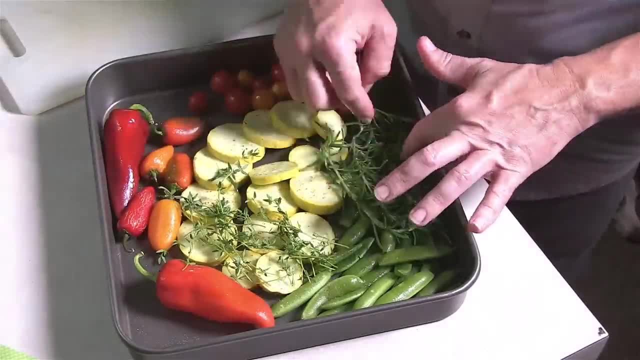 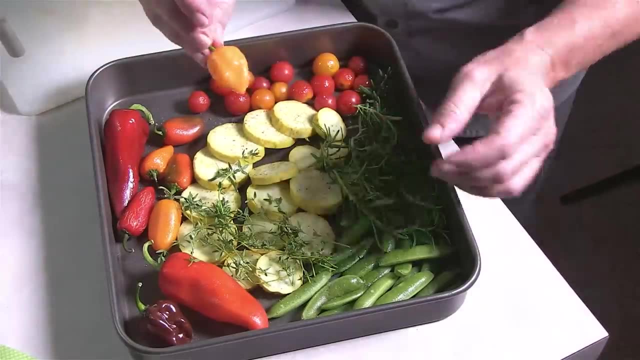 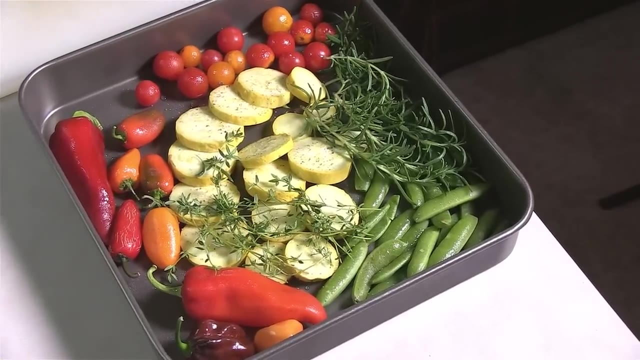 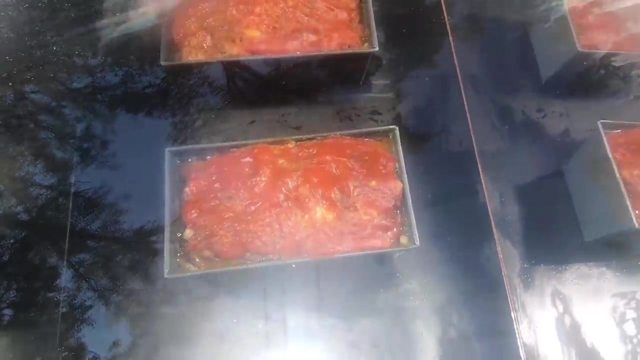 that I'm, that I'm cooking. I'm just going to use a lot of pepper. actually, the ones that I got here are just a small amount, and then I always else I'm Home wondering in one of these genetics also put in a my chocolate habanero and a regular habanero pepper. 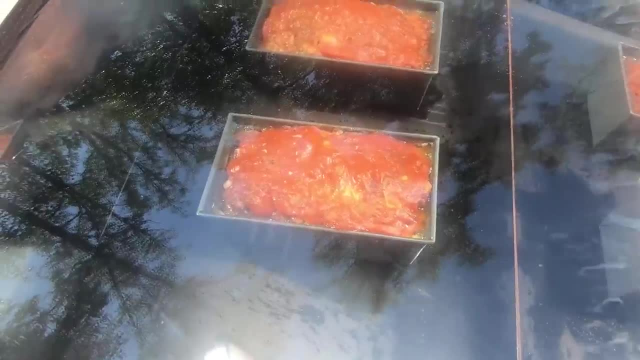 there's just some dishes that just really do taste better cooked in a solar oven and in comparison to a regular oven or microwave. I don't know if you can see this or not, but the juices are already bubbling in the little mini loaf pans. it's really quite hot in there. 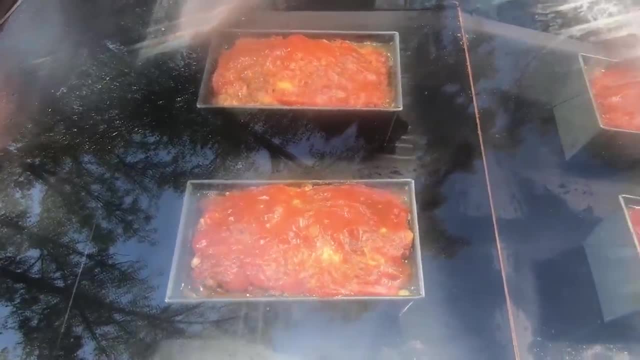 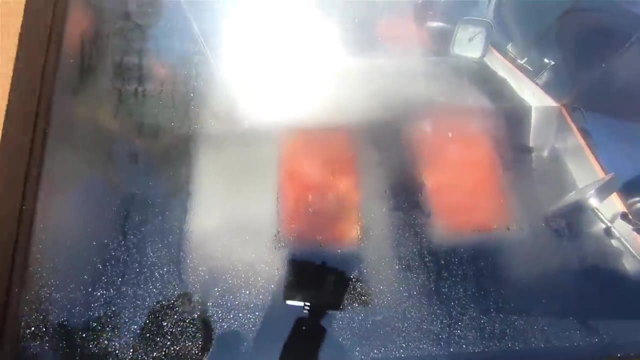 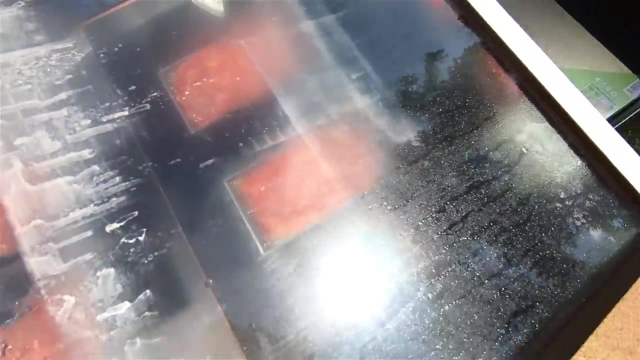 30lbs meatloaf already bubbling. it's really hot in there. it's probably about done. I'm gonna. I'm gonna let that sauce caramelize just a little bit more before I take it out. it's, it's looking really good. these were. these were actually with the 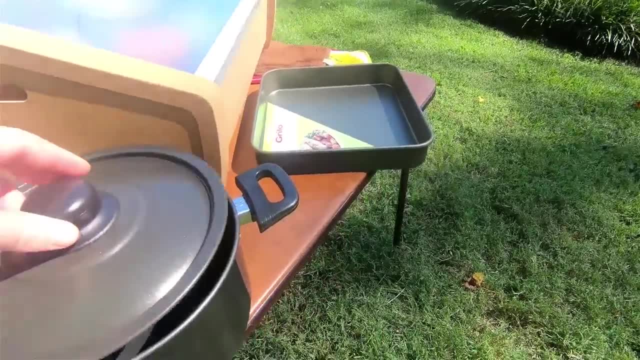 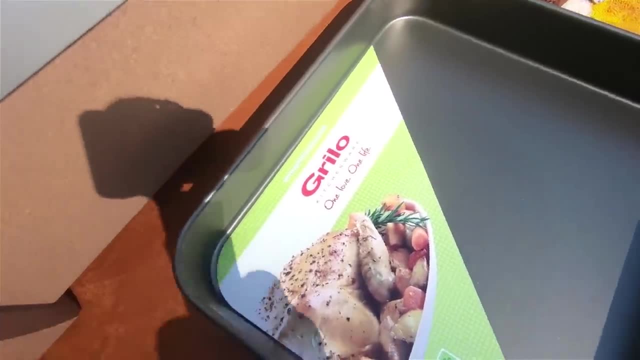 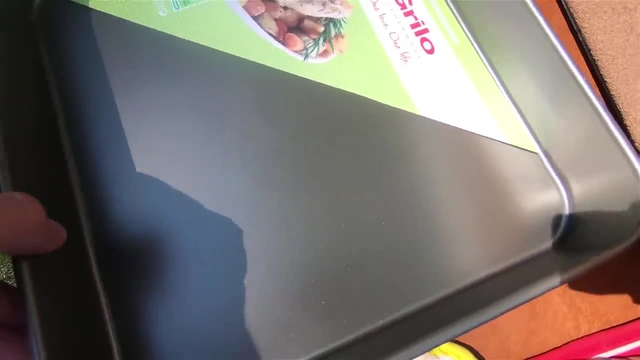 son of and this was kind of a nice surprise. these are really lightweight and they feel like they. yeah, they're definitely nonstick. it looks, says, by a company called grill on, but it's got a really nice nonstick finish to it and they're. they're nice and lightweight, but it's. 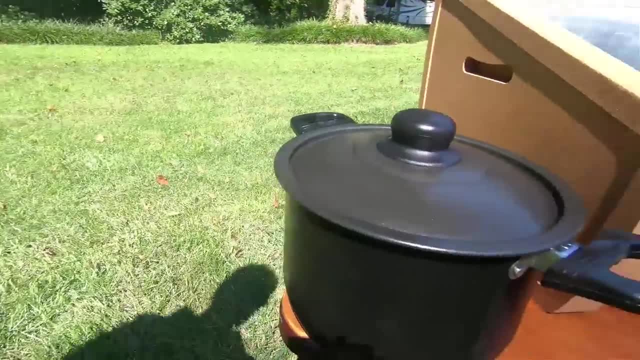 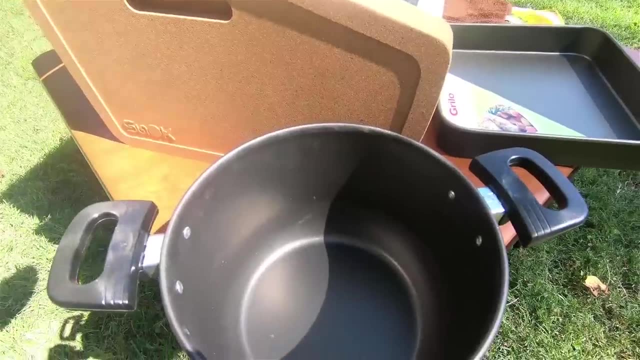 a, you know dark, dark metal, so it absorbs the heat really well. so I'm thinking that these are, these are gonna be perfect for, like you know, soups and stews, and you could, you could probably even put like a, like a whole chicken or like a. 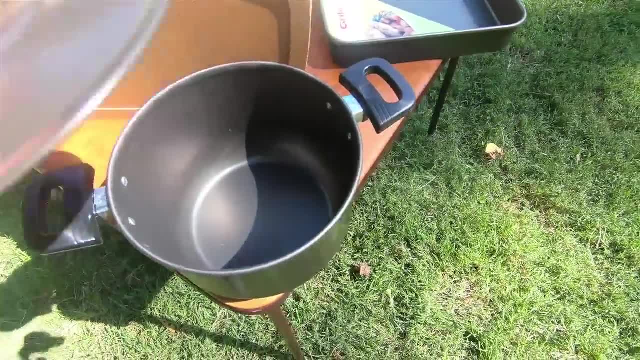 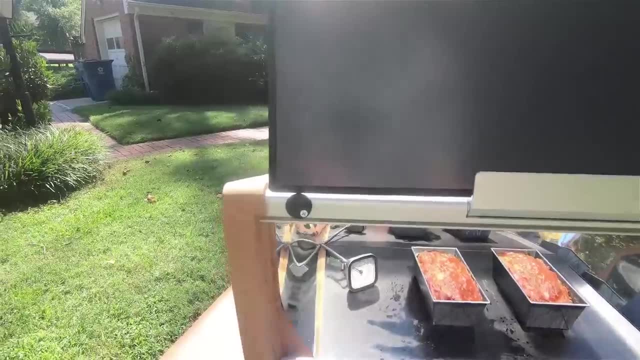 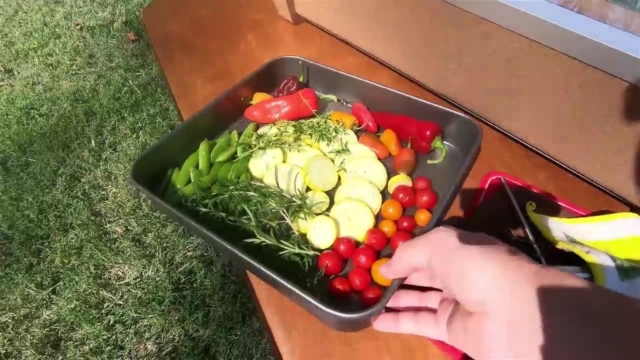 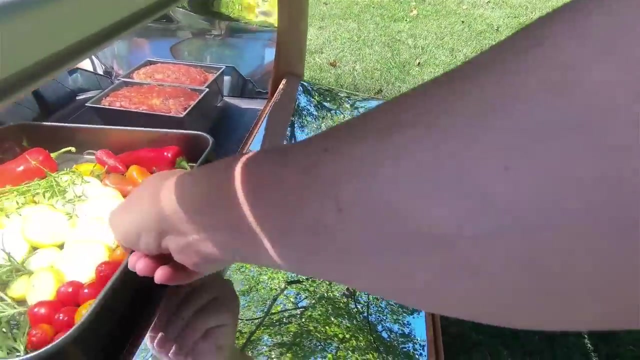 Cornish Hen in there That would easily fit in there. So I highly recommend trying this meatloaf and definitely the roasted vegetables like this in a solar oven. It's just so easy. I mean, you can just do other things. You can work outside in the yard. That's normally what I'll. 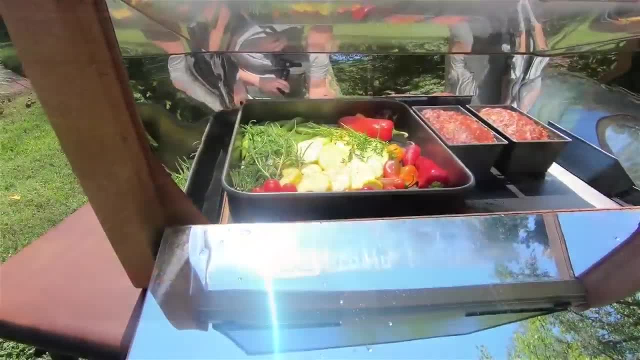 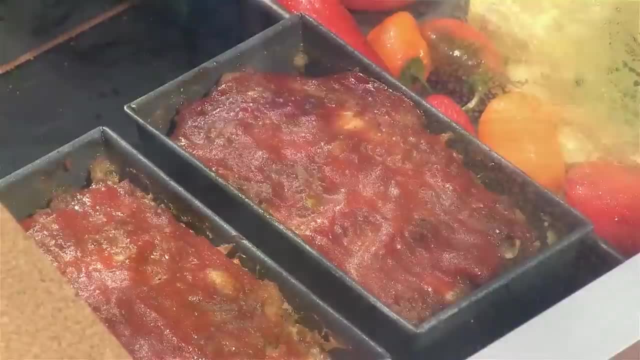 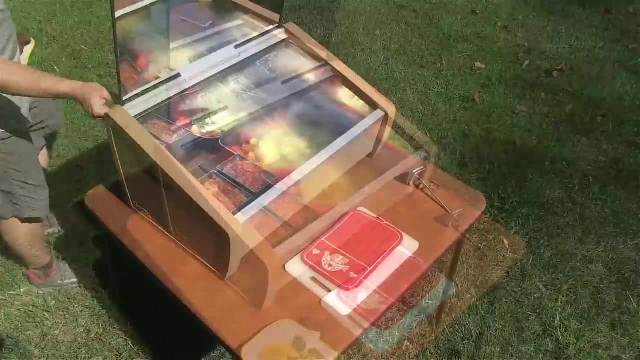 do while the food is cooking, And then you can just every 15 or 20 minutes just go and just kind of slightly rotate the oven to keep the sun angle correct for the reflection. But at the end of the day it's just so nice You can just smell it cooking and at the end of 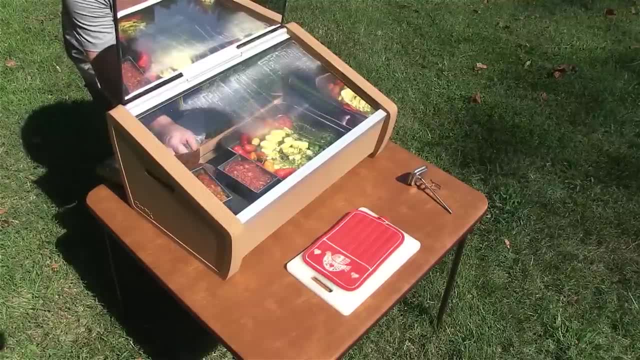 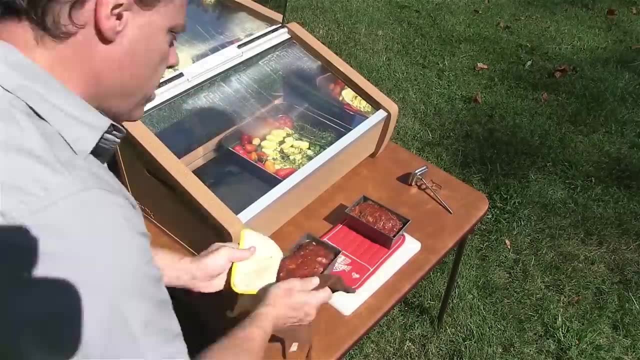 the day you've got a nice dinner and it's fairly healthy and it feeds quite a few people. I fixed a little extra because I was going to eat one for dinner and then probably not eat another one, Probably lunch and maybe even dinner for the next day. So I fixed- I fixed two of 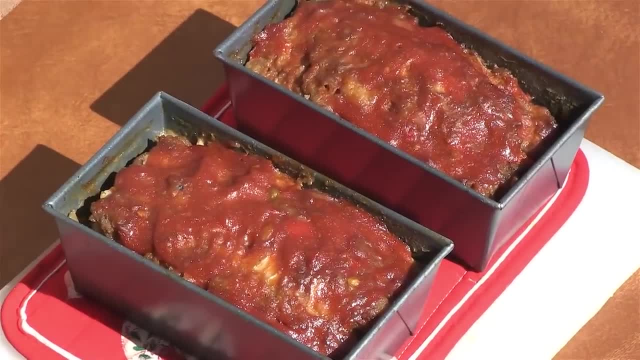 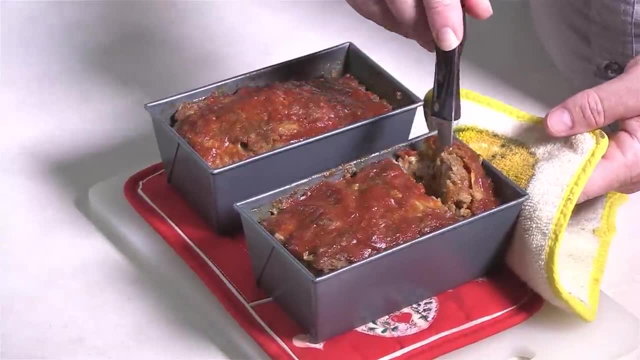 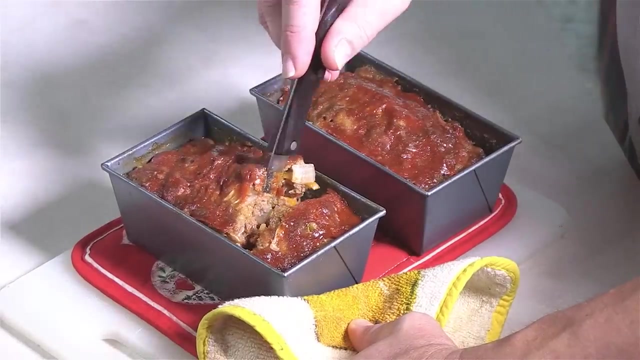 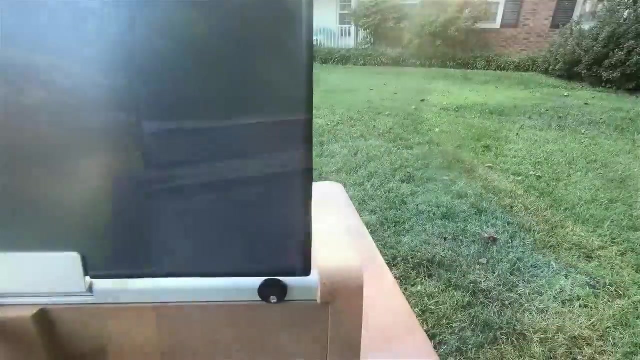 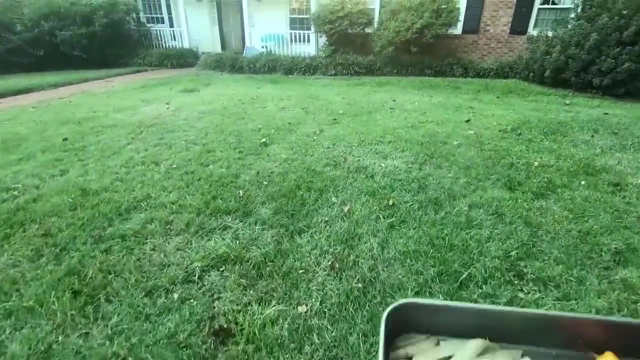 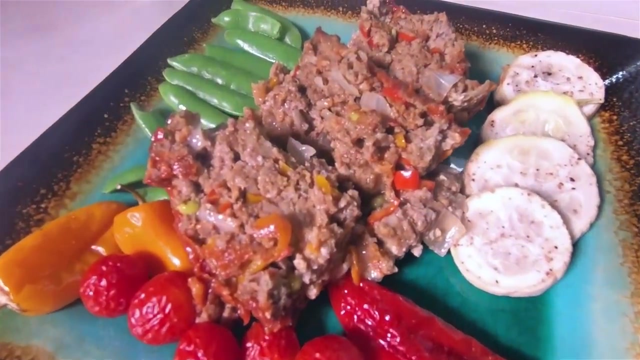 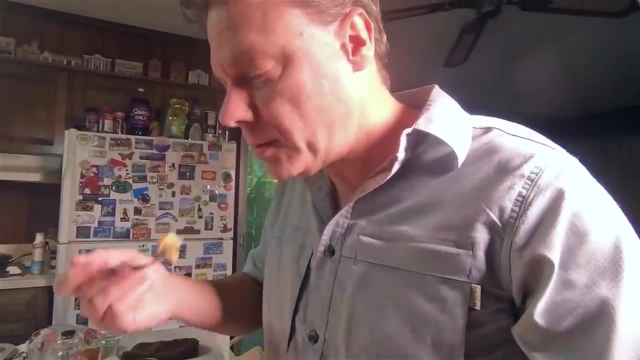 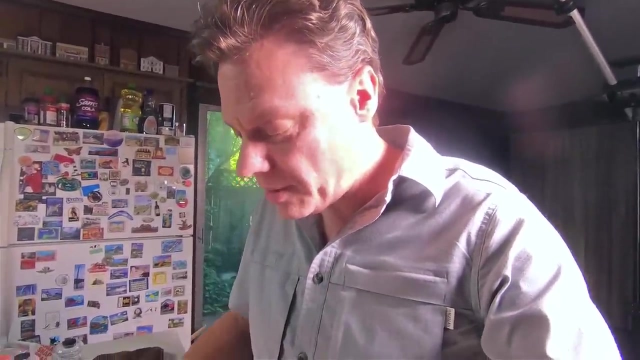 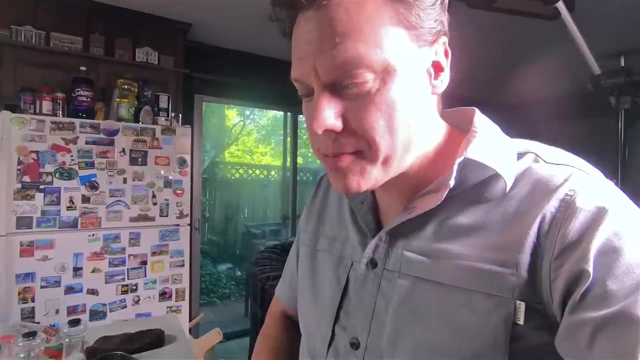 them. But it is a wonderful oven. I highly recommend it, And so I might actually try to try to buy the the small version. But yeah, you want to try to be starting from the small version of a regular. you go to the kitchen and make your own and you can have. 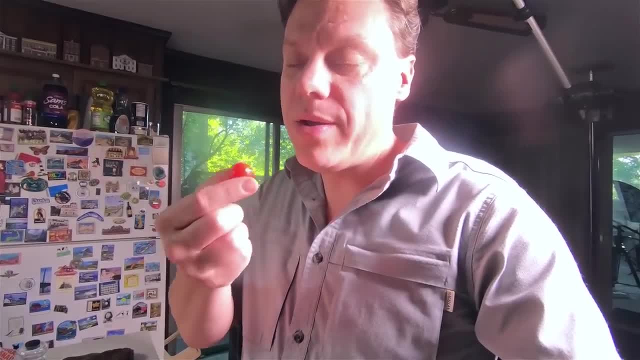 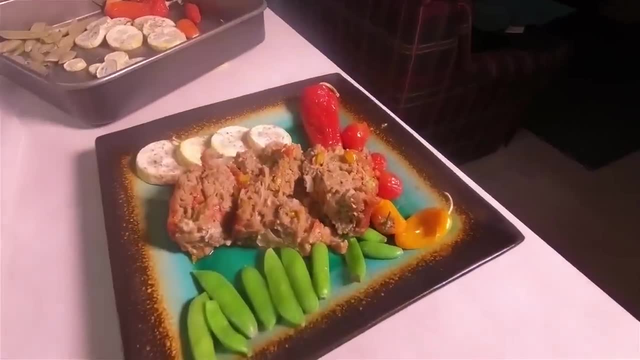 dinner or lunch, or dinner or lunch. you can do that by yourself, Or you can just get the food on your own. The only thing I'm going to tell you how to do is to just to make sure that you're on your own, Okay.